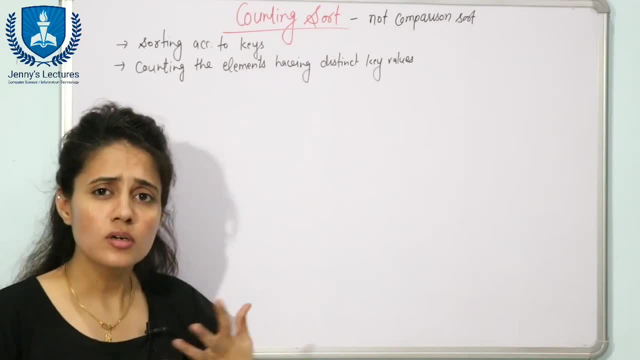 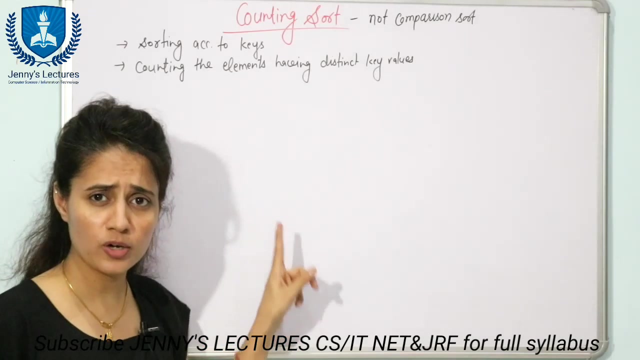 see, as the name suggests, counting. so you are going to count the number of elements having having distinct key values, so fine, or you can say different key values. now, what is this key value? how we are going to count the number of elements, how we are going to sort. we are going to see this with the help of an example. 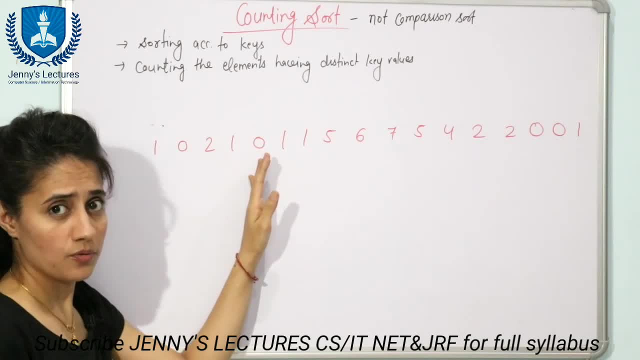 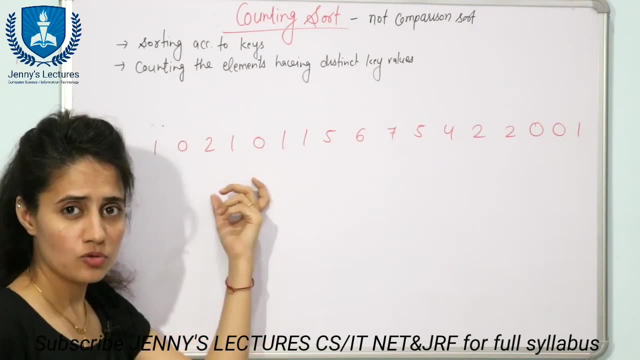 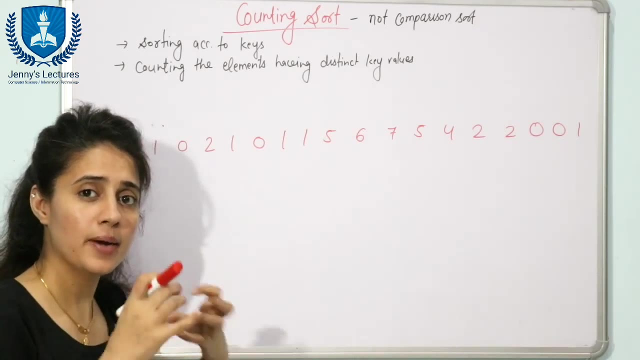 so see, let us suppose you are given this array, fine, and you are going to sort this array. see, although you can, you can apply that any comparison: sort, merge, sort, quick sort and the time complexity for that, the best time complexity would be n log n. you cannot get better than n log n. 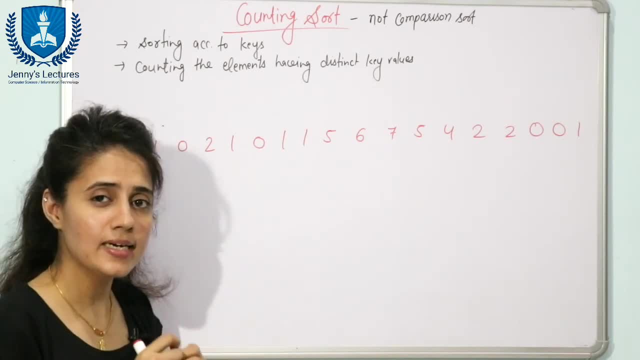 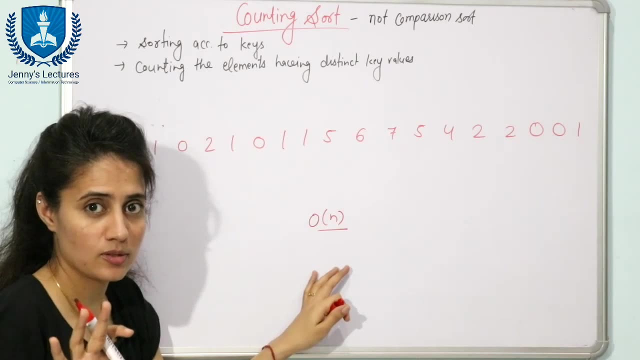 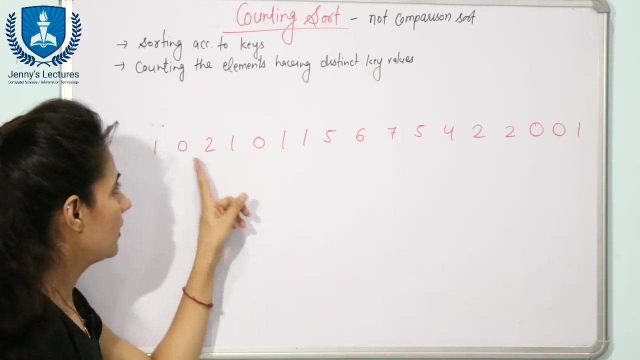 but how we can sort in linear time. you can say order of n time. is it possible? sometimes it is possible, see, sometimes we are going to see the time complexity of this counting sort and how we are going to sort this. so see, here, in this array zero is one, two, three, four, four times one is also. 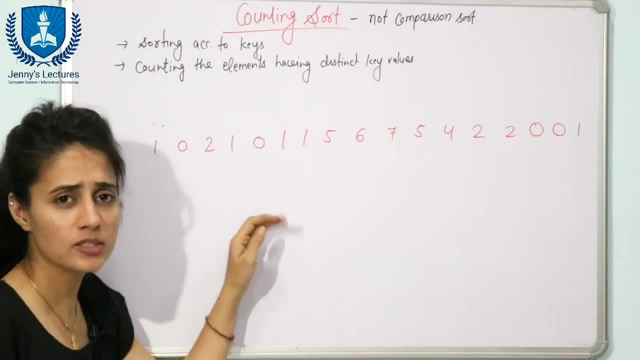 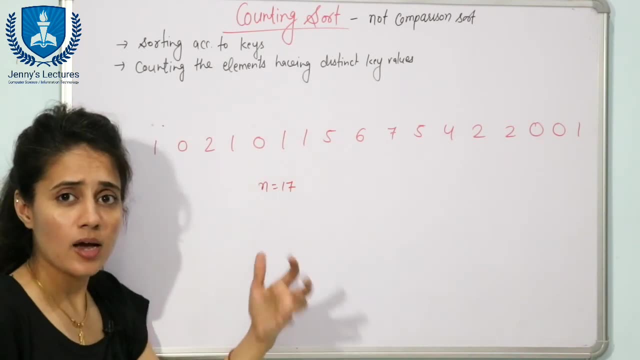 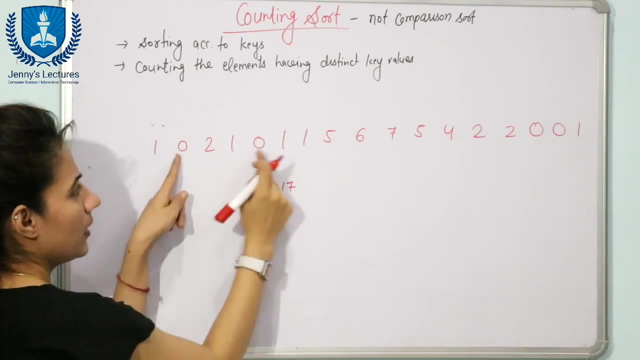 repeated. two is also repeated, i guess five is also repeated, something like this. so here, total number of elements are seventeen. fine, and all the elements are in the range of see from zero to zero. to see: minimum element is zero. maximum element. find out the maximum element in this. 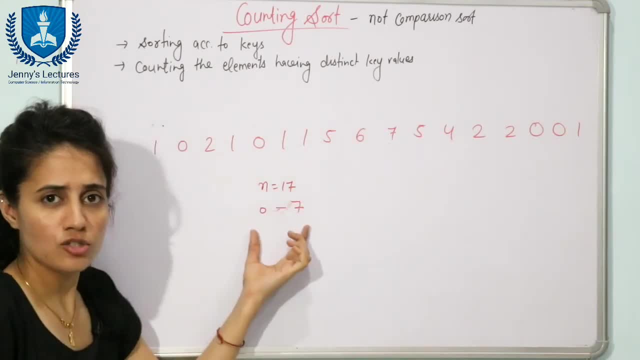 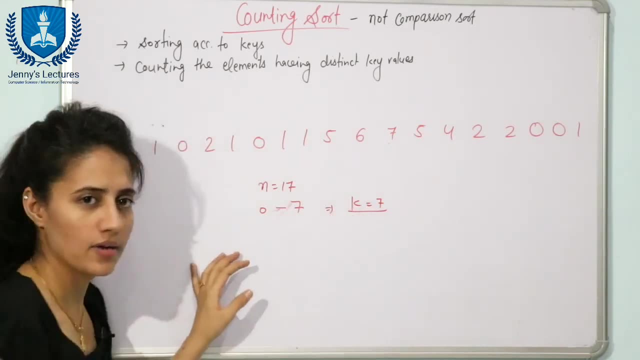 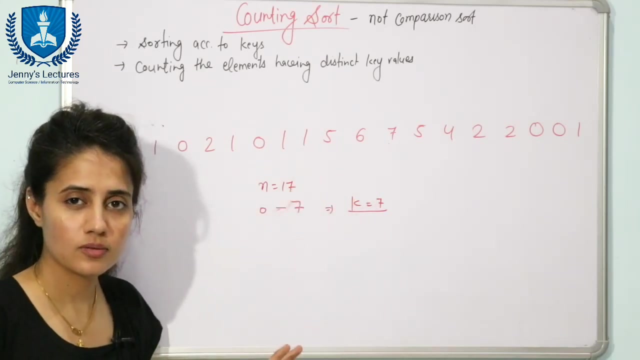 array maximum element is, i guess, seven. so range is from zero to seven. fine, so you can say here k value is seven. so here you can say we have an array having k different elements. right, and maybe in this array values can be duplicate, values can be there. so how? 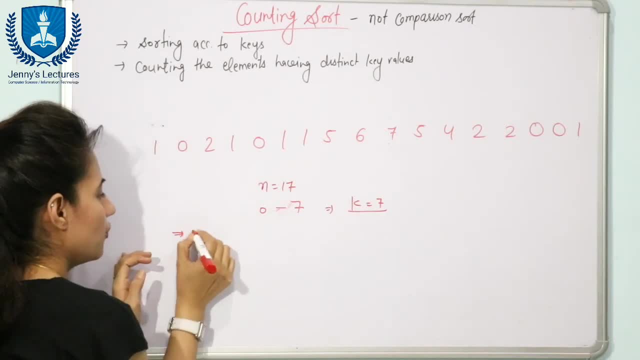 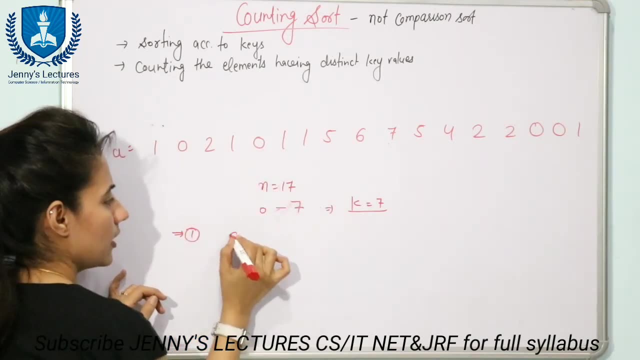 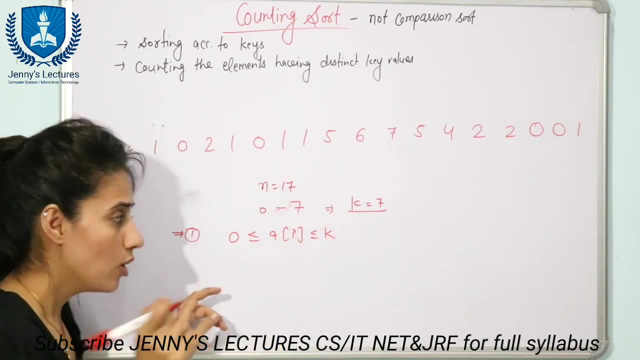 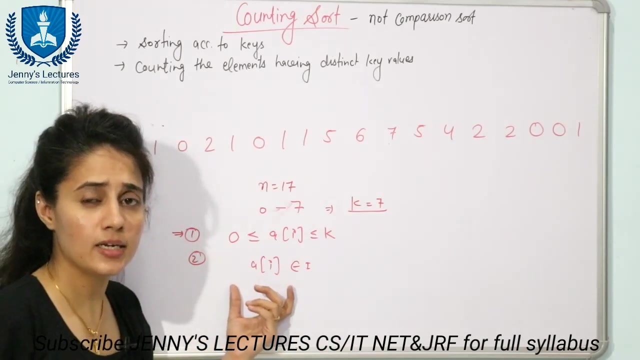 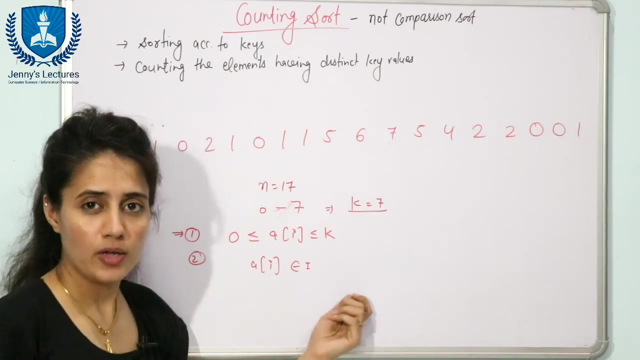 to sort this array. so here the situation is. first case is first case is suppose the array name is a, all the elements in the array would be in the range of zero to k. fine. or second case: may be this notion or function to be this unit. we say that one value of a nucleotide ella. 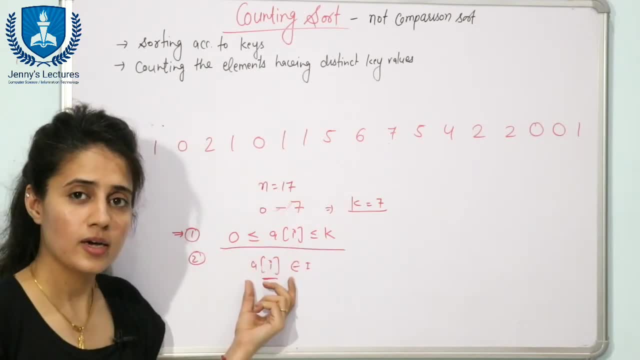 refers to this empty square in the question. are all all the elements belongs to any integer, maybe zero, negative, positive, very large integer, very small integer, something like this, with k different values. fine, so we are going to check this case. so here for this case, we are going to apply another. 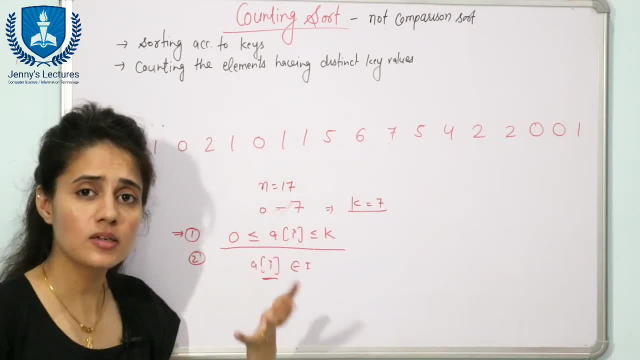 sorting algorithm, because here values can be negative. so this counting sort- we will discuss that- will not work on the negative values. fine, so condition is here: the array should contain no negative values and the values should be in the range of 0 to 50? to k. somewhere in in some numericals you are given this k value in the question only. but 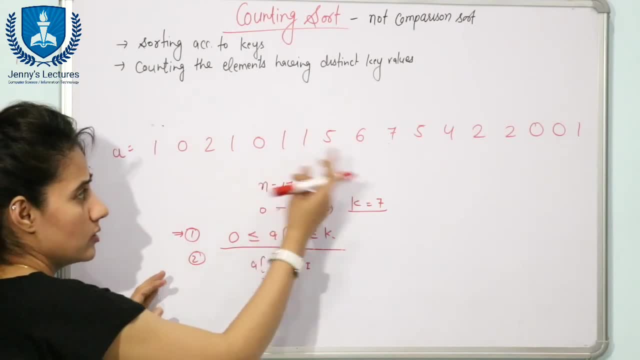 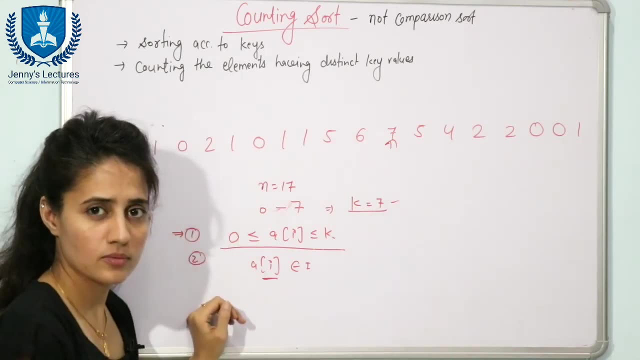 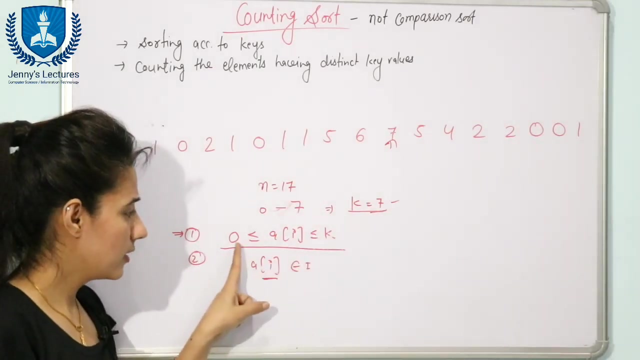 somewhere it is not given so you can find out k value just you. just you check out the maximum element in this maximum element is 7, fine, so k value would be 7, right, and range would be from 0 to k. so first of all, we will discuss this case- range would be from 0 to k- with help of an example. 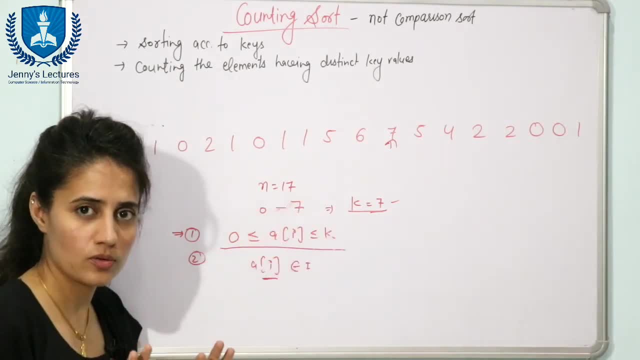 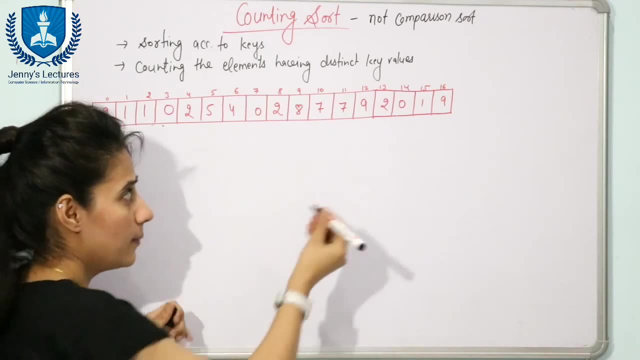 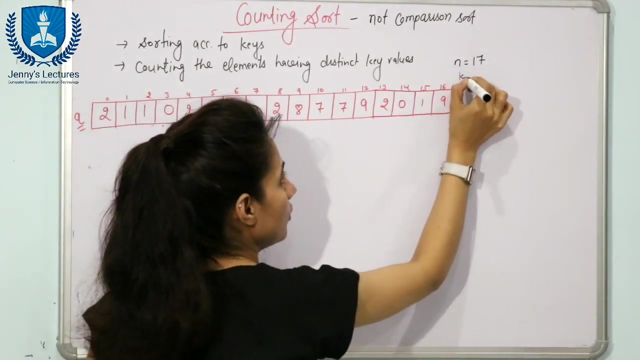 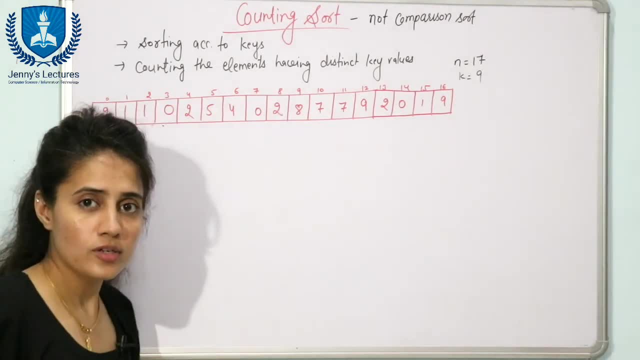 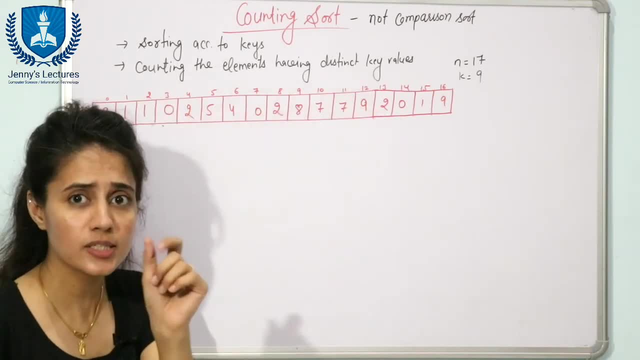 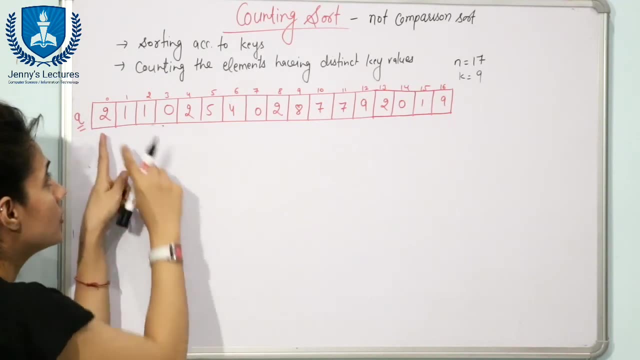 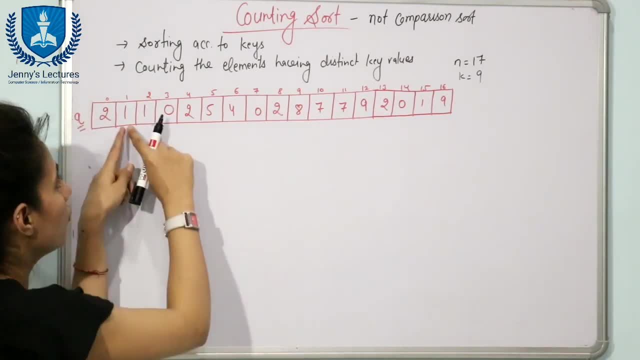 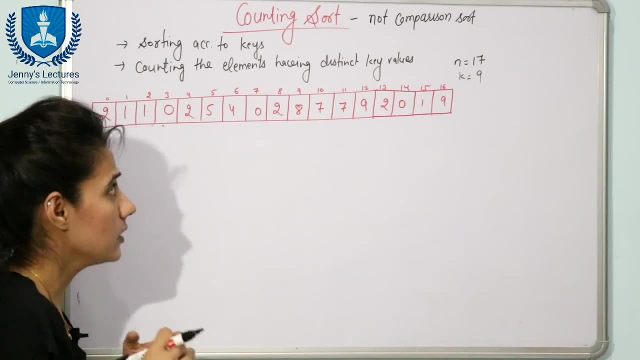 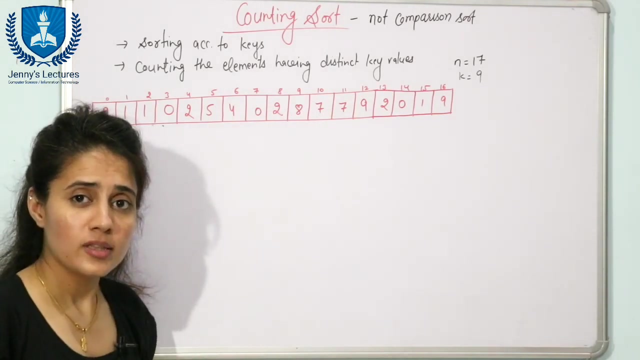 5, 5. How many times one is there in this array? one, two and three, three times. like this, you are going to count the elements, fine, and after counting, obviously you are going to store those elements in somewhere. so for storing that count, we are going to take another. 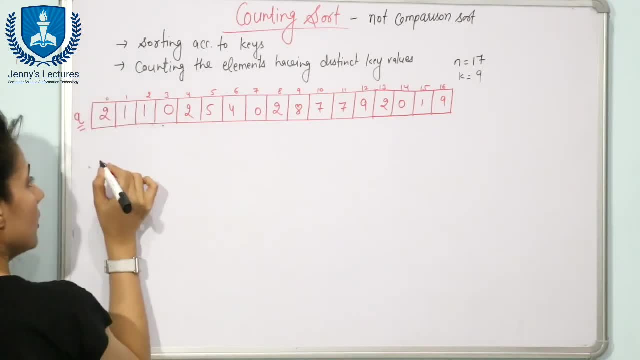 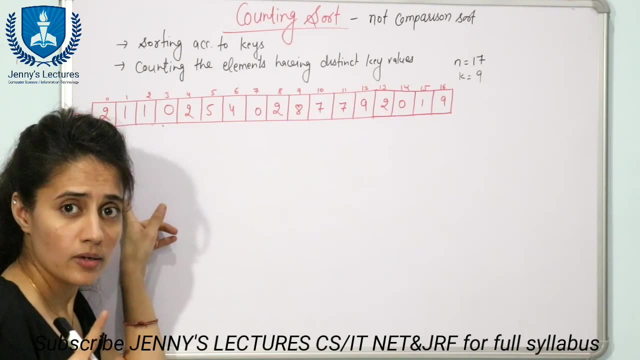 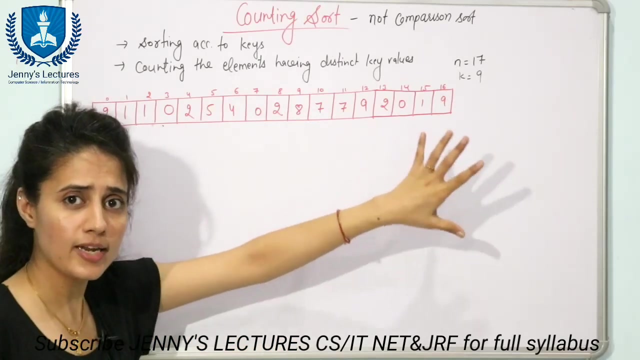 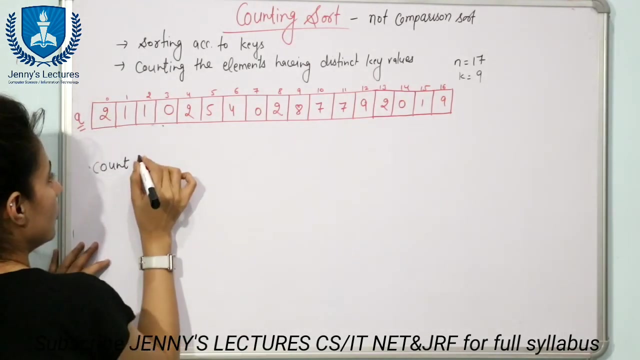 array and i am going to take the name of the array as count right now. the size of this count array would be this: k plus 1. so 9 is there. see, range is from 0 to 9, so 10 elements would be there. range, this size would be k plus 1, or you can say range plus 1. so let us suppose this array is there. 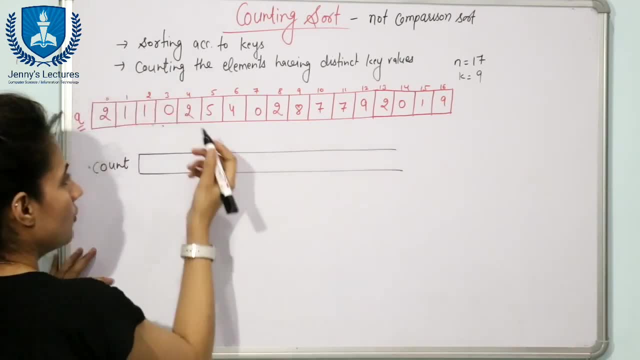 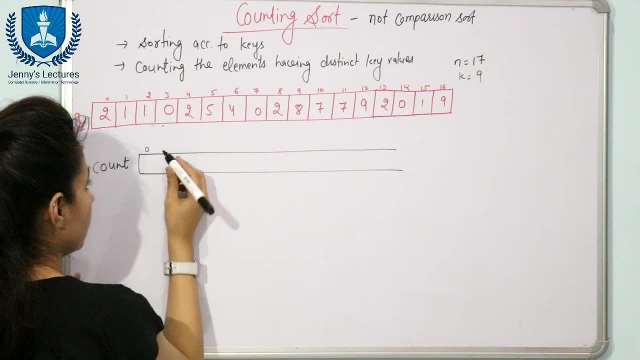 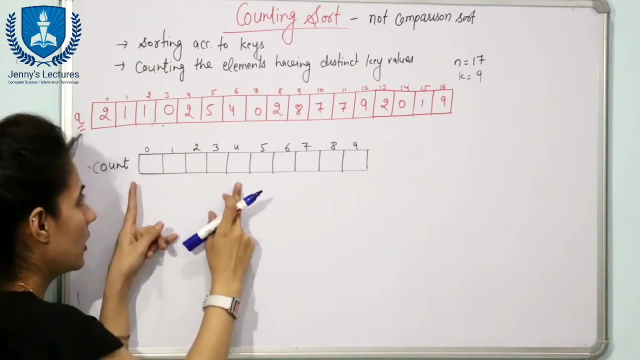 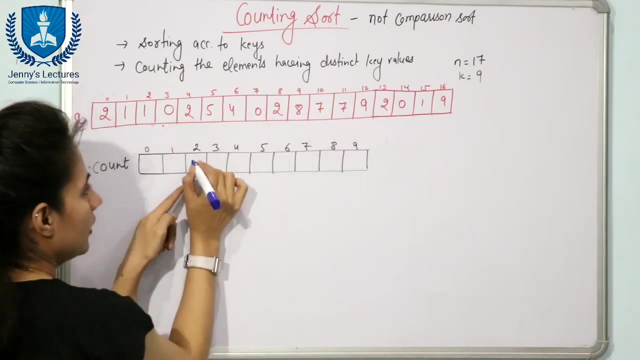 another array. so index would be from 0 to 9, same as the range of this array. given array. now we are going to count the frequency, or counting the elements having distinct key values, c. so see what should be there in this count array. the key value is 2. this 2 is how many times 1, 2, 3, 4. so here we should have 4, see 1. 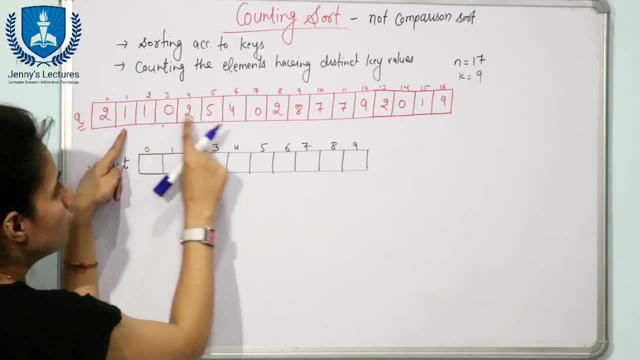 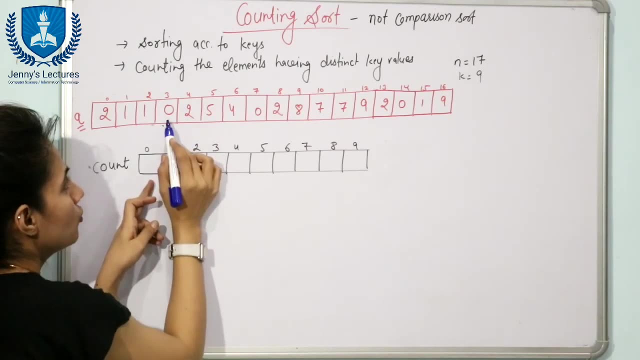 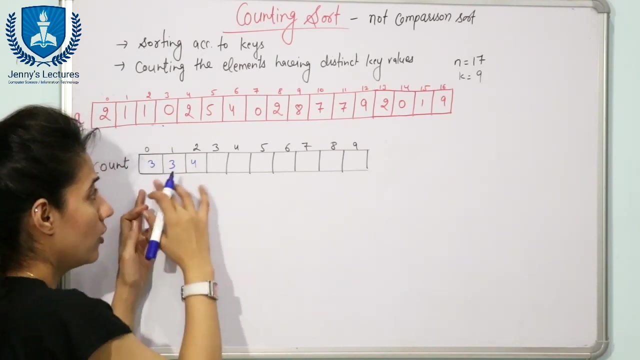 the key value is 1. 1 is how many times? 1, 2 and 3. so here 1 is there and this is how many times? 3 times, and next, 0. 0 is how many times 1, 2, 3, 3. like this, you will, you, you are going to fill this. 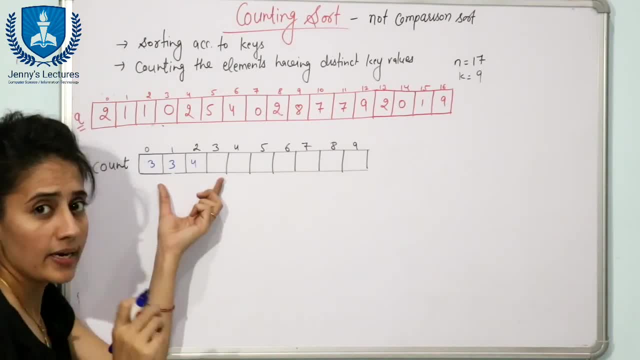 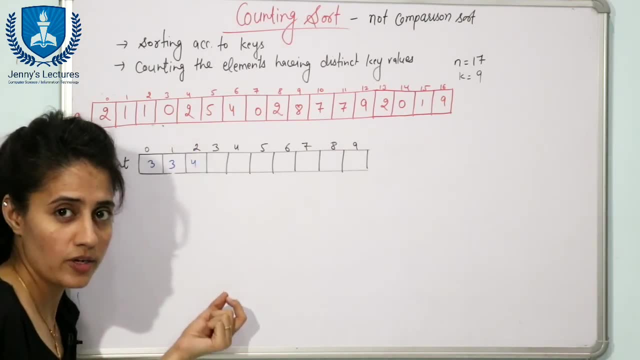 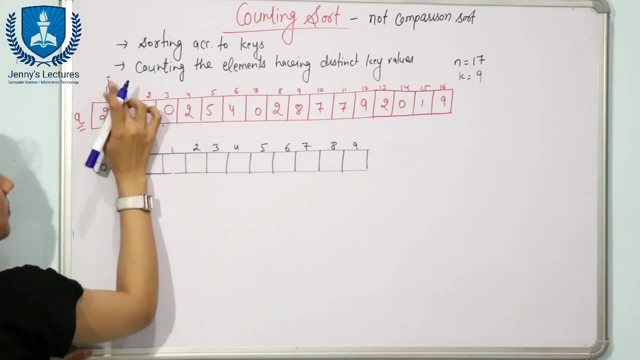 array. but now we will see how we are going to fill this array, actually how we are going to write down 4 here, how we are going to count the number of elements, fine, how we are going to write down the code c. first of all, we are going to take one variable, i fine. here the value is: 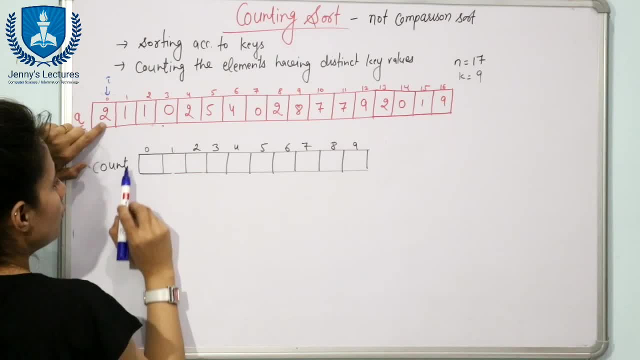 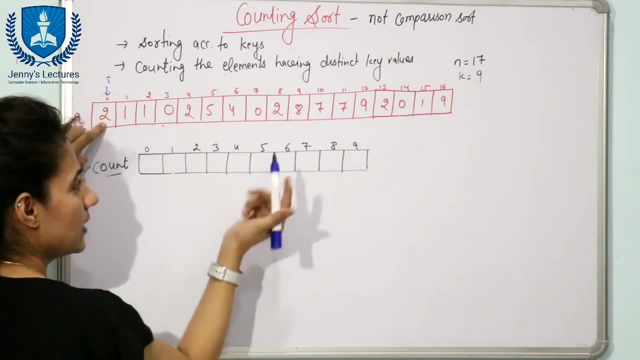 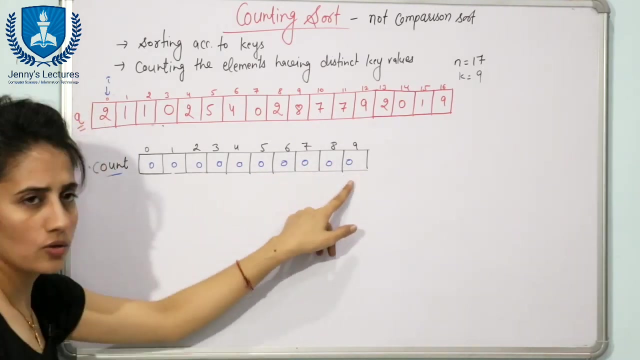 3, 2. right, so the value is 2 in this in this count array. go to the index 2. this is the index 2 and at starting, the value in this count array would be 0. you are going to initialize this count array would be 0, all the values, right, fine, now see this: 2. go to the index 2 and. 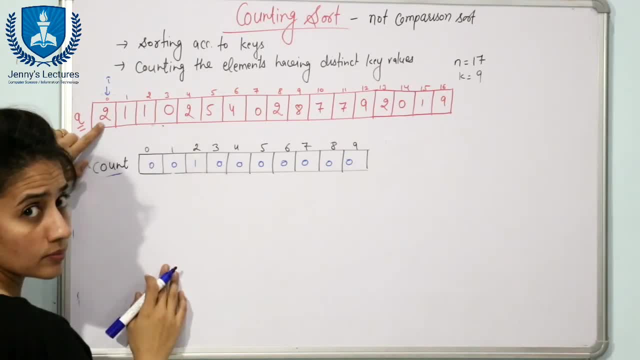 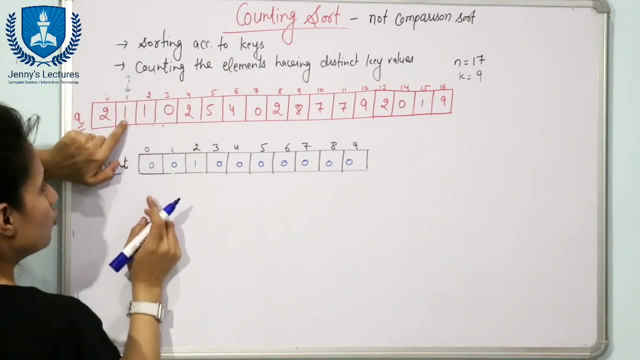 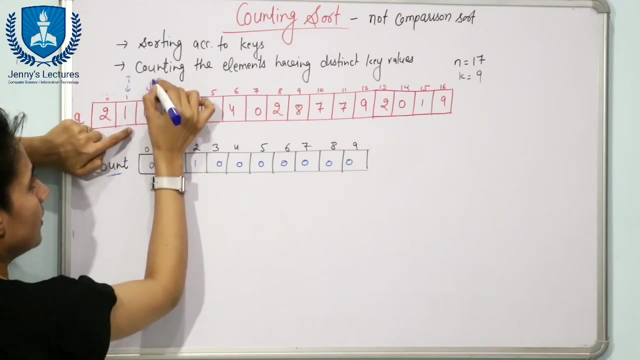 increment this value. now it becomes 1. you are going to add 1. now i would be at 2 this place. you are going to increment this. i now. here value is 1. now go to this index 1 and increment this value. this is now 1. now again increment i. value is 1. again go to the index 1. 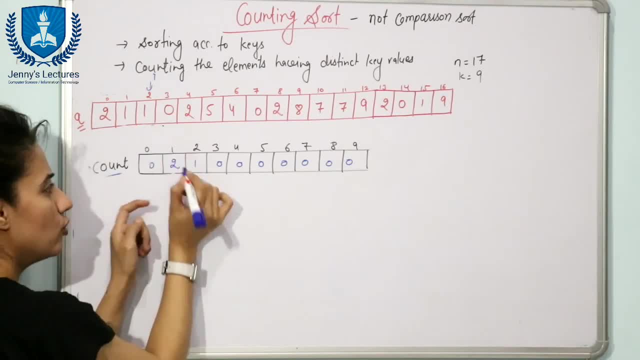 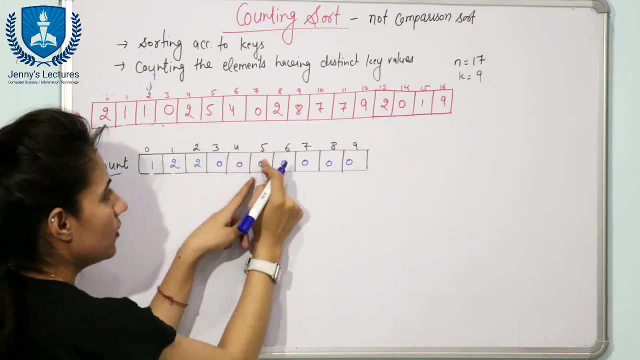 and increment this value. we have 1, so after incrementing, the value becomes 2 now. next is 0. go to the 0th index. increment this value 1. now. next is 2. go to the index 2. increment this value. that is 2. next is 5. go to the index 5. increment this value. next is: 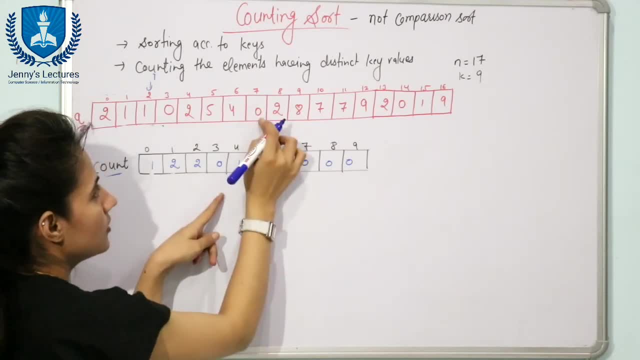 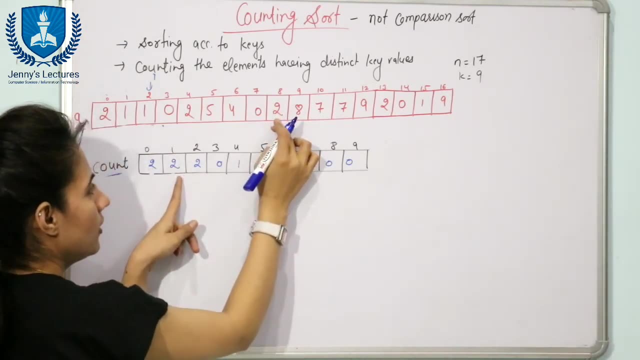 4. go to the 4th index. increment this value. next is 0. go to in 0th index and increment this value 2. next is 2. fine, go to index 2 and increment this value. that is 3. next is 8. value is 8: fine. 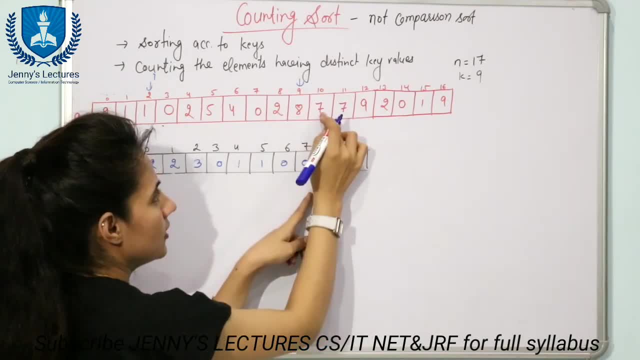 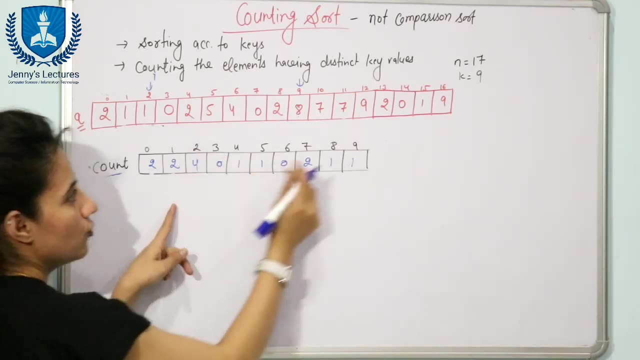 so go to the index 8. increment this value. next is 7: index 7. increment this value. next is also 7. go to index 7. increment this value again. next is 9: go to index 9. increment this value. next is 2: go to index 2. increment this value. that is 4. next is 0. go to this 0th index. increment this value. 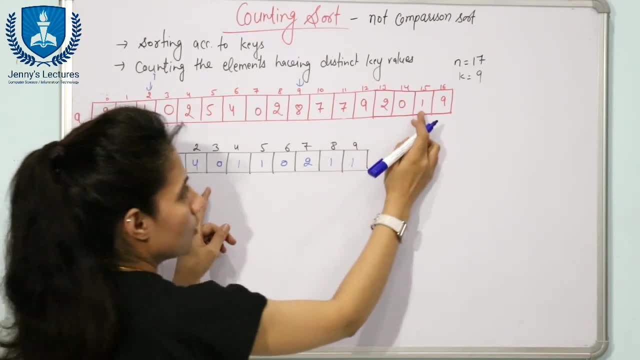 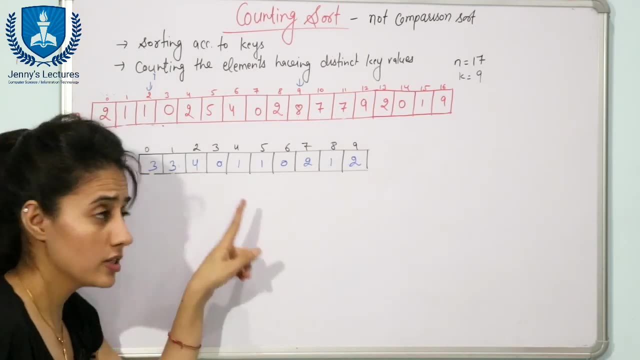 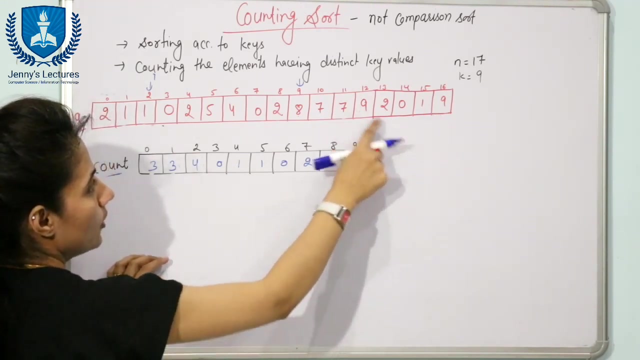 1. go to index 1. increment this value. then last is 9. go to the index 9. increment this value: 2. fine, this is how we are going to fill this count array. you can check out this: 9 is how many times 1 and 2. this 8 is how many times only 1. fine, how we are going to write down the code for. 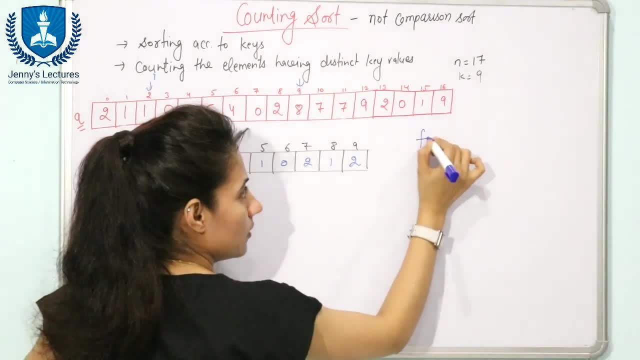 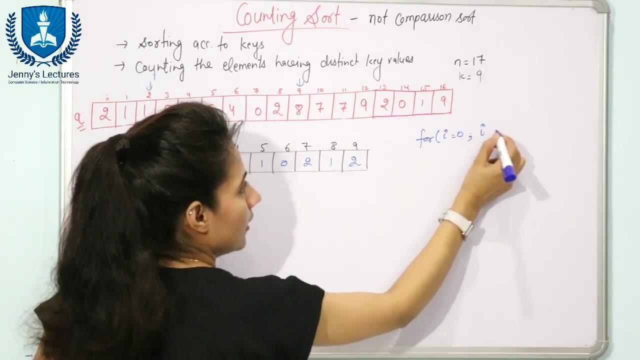 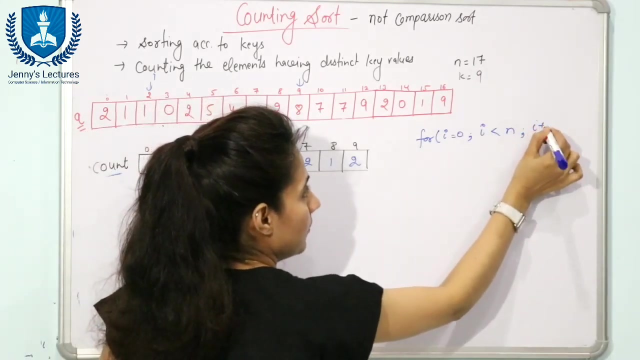 this. see, we are going to take one for loop. we are going to take one variable, i. i would be started from 0 and i would move till here. less than n, or you can say less than equal to n minus 1. n is 17 and i plus plus. now how to fill this count array? you are going to write down code for. 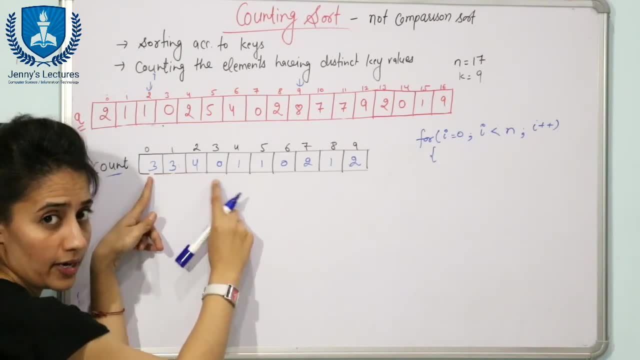 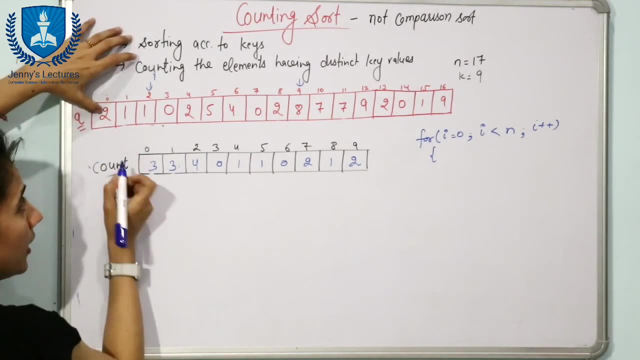 that you are going to increment this value count array value. fine, see first of all what you have done. you have just checked this value, that is 2, and you have gone to the index 2 and then increment this value. fine, so how we are going to access this value. array name is a. 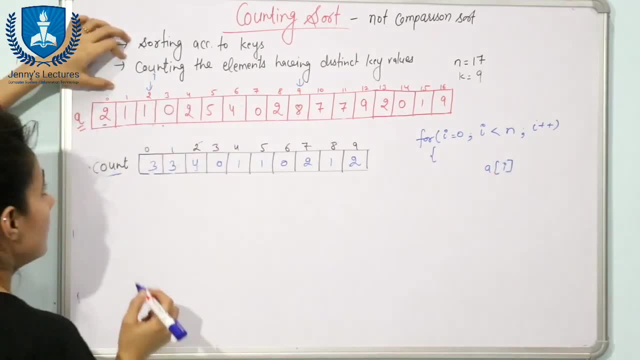 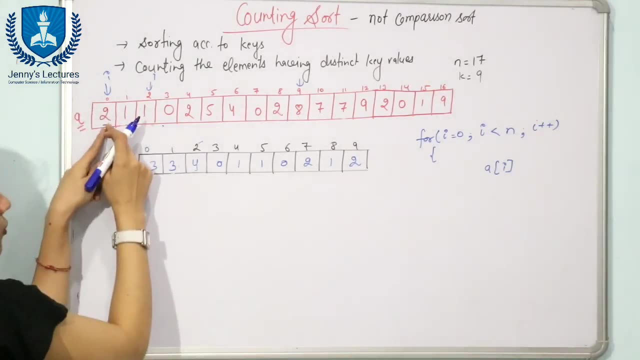 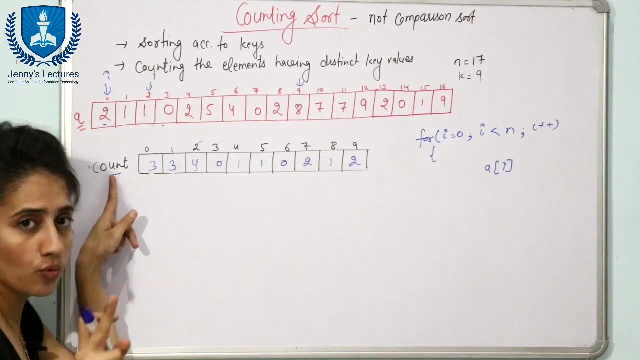 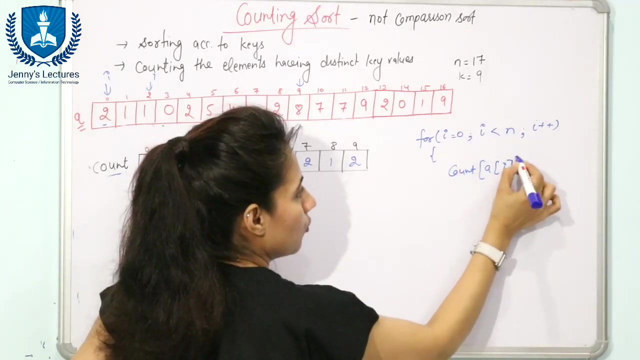 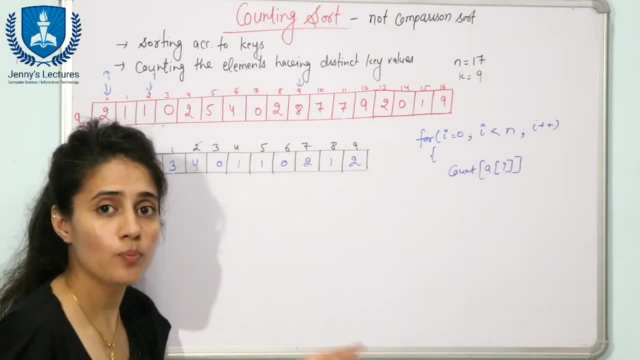 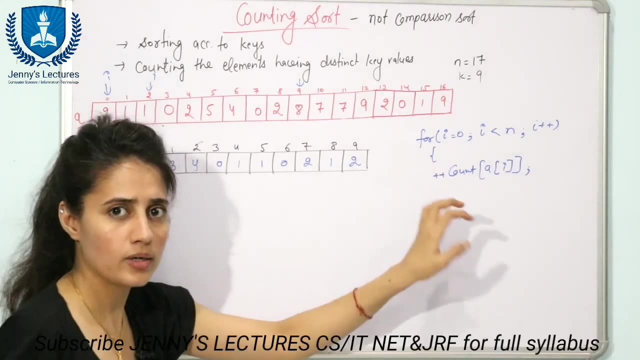 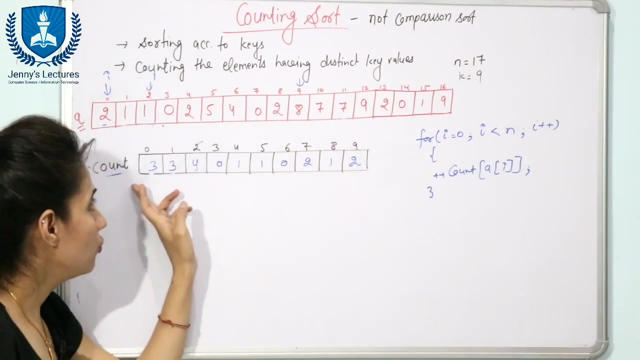 here you will write count brackets, and now i will do plus plus. so here you can write plus plus number numbers, or here you can write plus plus post increment or pre increment. in this case, both will be same. this is what you have done at starting. when you are going to take this array, you are going to initialize this array. 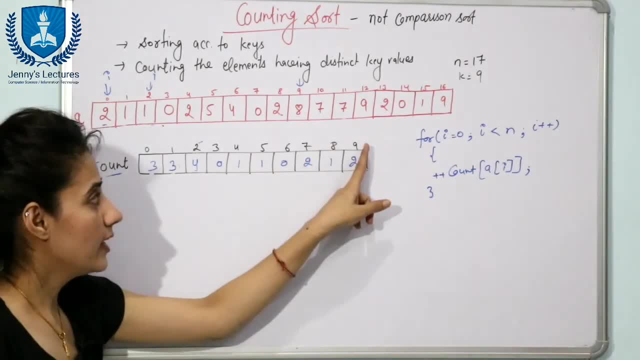 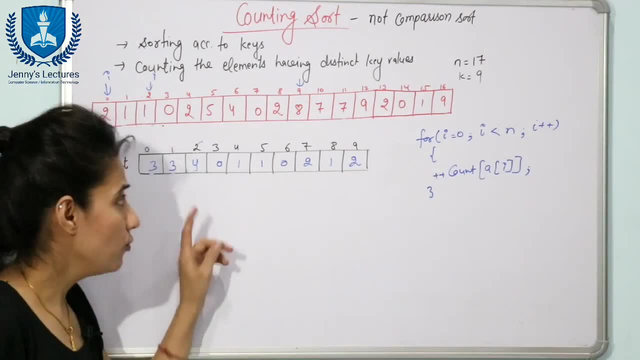 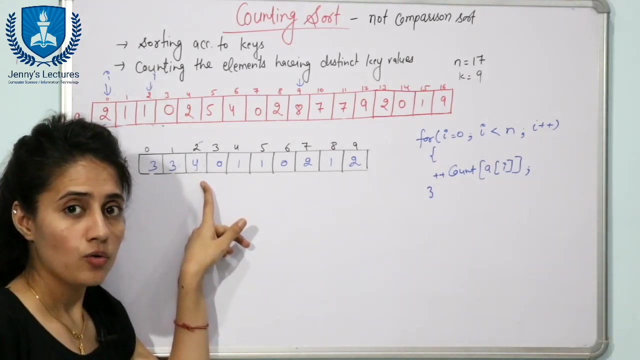 with zeros, for i is equal to 0, i less than equal to k, k and count of i is equal to zero. so now, next step is: now you have. you have counted the elements, the frequency of the elements, fine, but now you are supposed to find out the actual position of these elements in the sorted 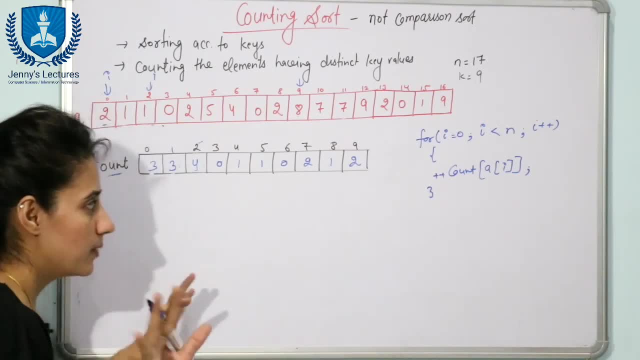 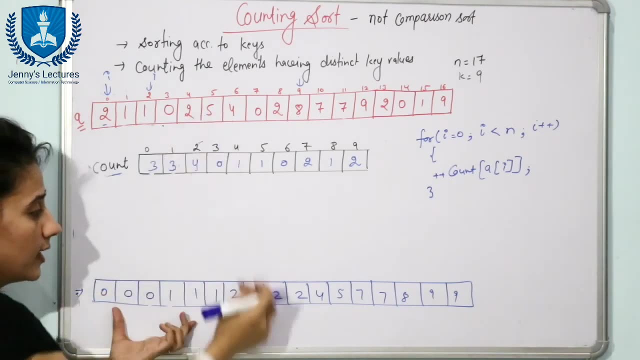 array: see after sorting. the array would be something like this: see after sorting: after sorting array would be something like this: fine, this is unsorted array. this is sorted array, right, so this 0 would be from 0 to 2. the index would be from 0 to 2. fine, first three position. 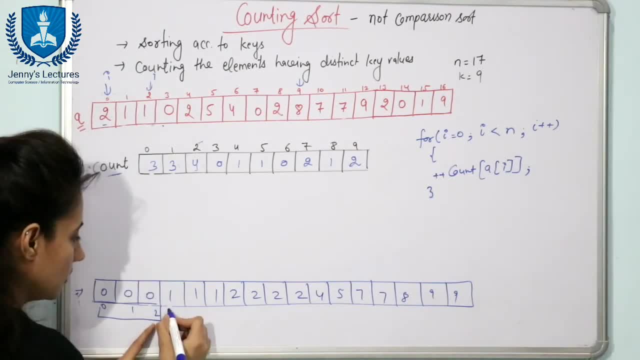 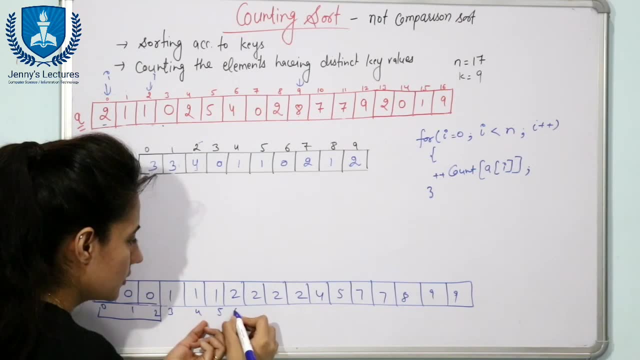 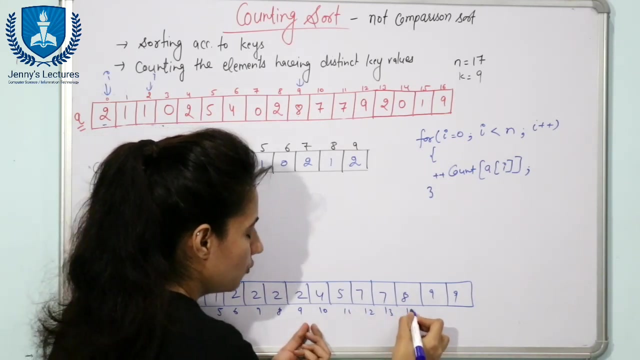 for 0, then position for 1 is 3, 4, 5. these position 3 to 5. position for this 2 is 6, 7, 8, 9 from index 6 to 9. this is 10, 11, 12, 13, 14, 15 and 16 for 9th. 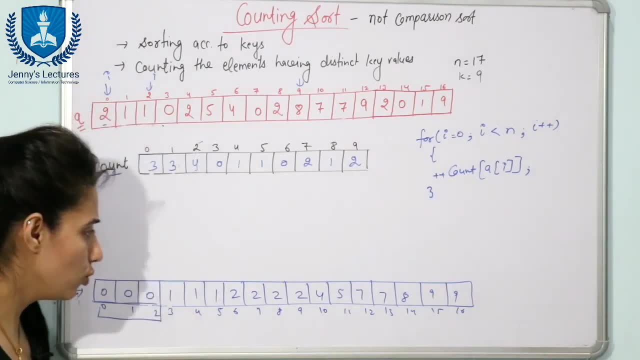 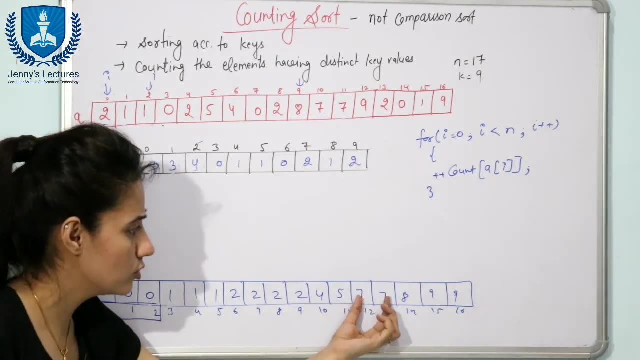 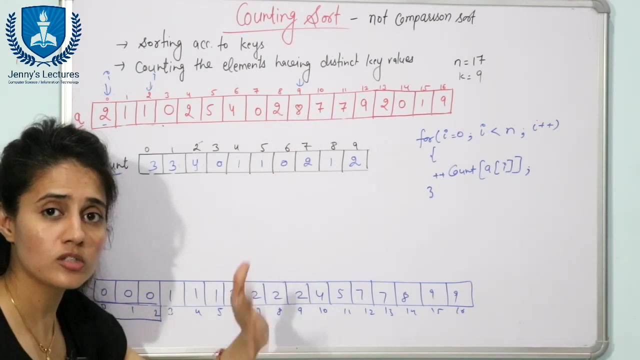 the position would be 15 and 16.. now, how you will come to know that the position of 1 is from 3 to 4, from index 3 to 4? how will, how you will come to know that the position for this 7 is? because here, from here, you can say that 7 are two times in this array. but what is the position? 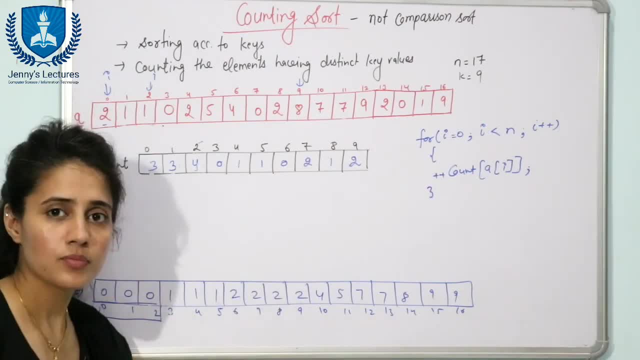 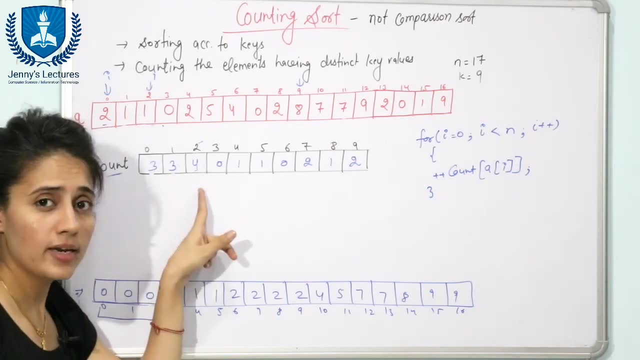 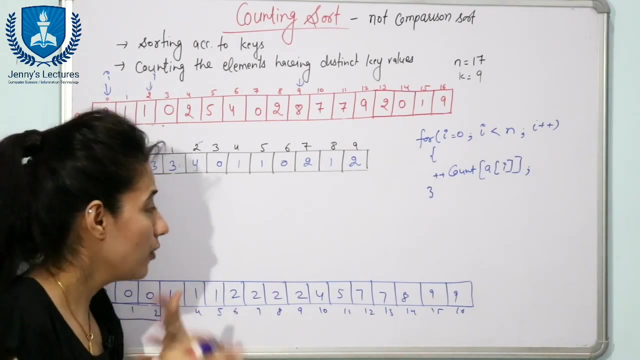 in this sorted array at index 12 and 13.. so now we are going to update this count array, fine, such that this, this count array, contains the actual position of the elements. fine, see how we are going to do that. you are going to update this. 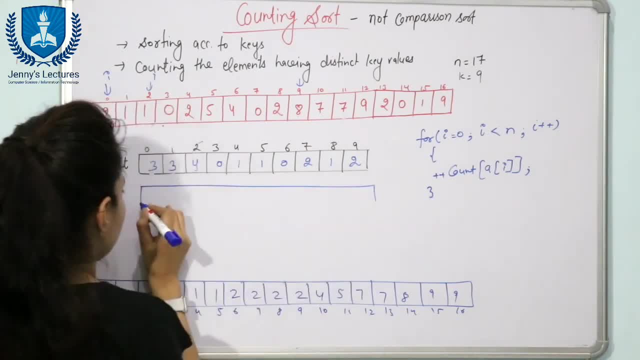 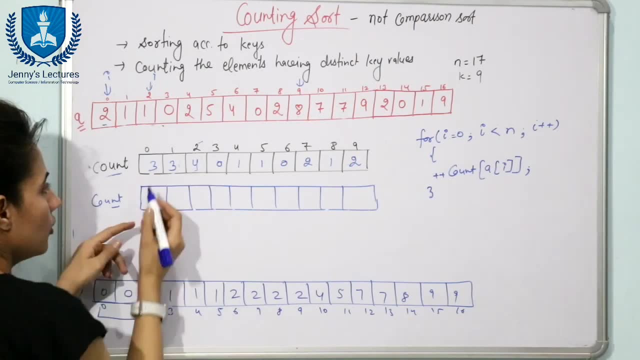 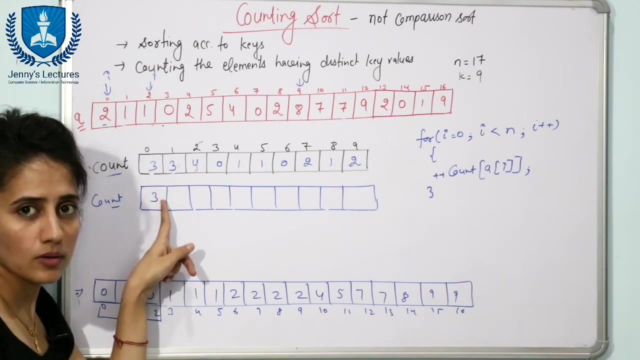 array. i am going to update this count array. this is same count array. we are going to update in the same array. fine, see first. first value would be as it is, the value at index 0. that would be as it is. we are going to start a loop from. 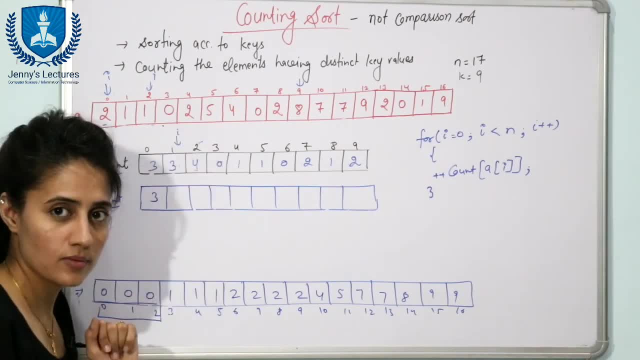 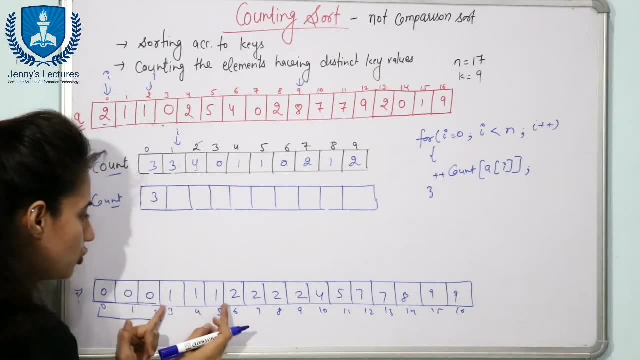 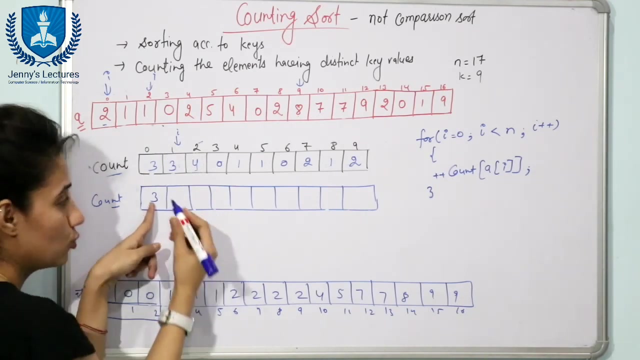 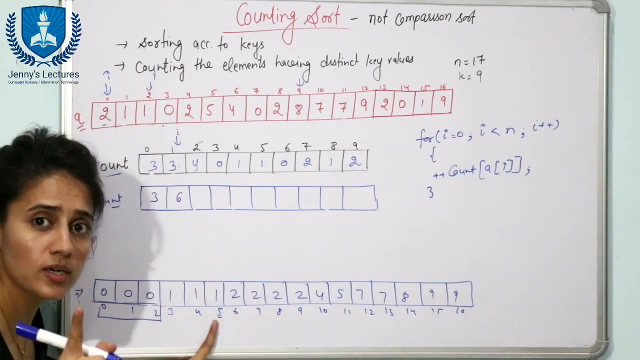 here only from the first index. fine, after these three zeros, after three zeros for next three, for next three positions, one would be there. fine, so the position of one would be see after these three zeros. so three plus three, that is six, up to six, see index is five, but position is six. one, two, three, 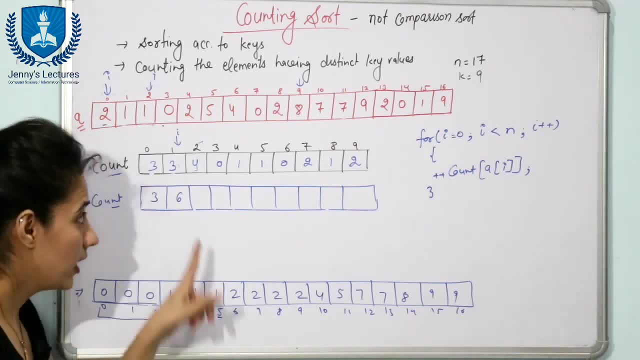 four, five, six, right, 6.. here we are going to. we are going to take the count now. that is why we are going to take the 6, how we are going to find out this position 5: i am going to tell you later. fine, now after. after 1: 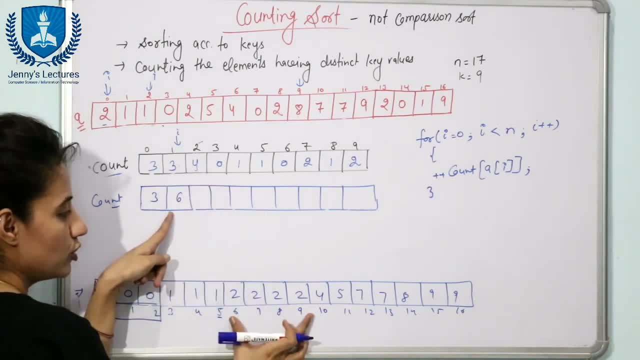 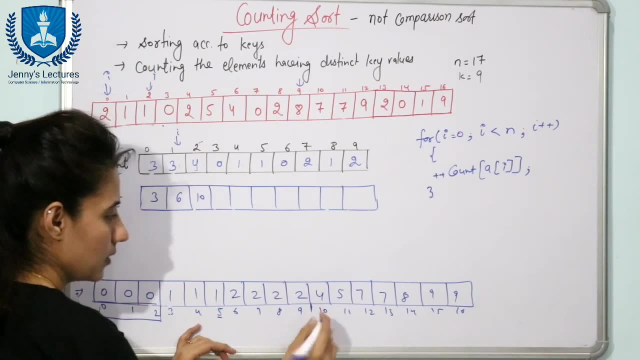 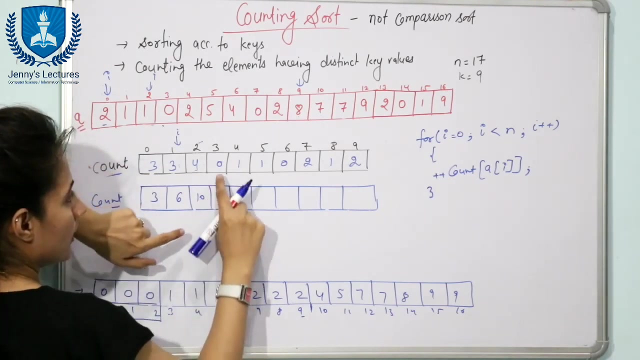 after 1, next 4 would be 2.. so position of this 2 would be 6 plus 4, that is, 10 till 10. here see: index is 9, but position is 10. this is how we are going to update this arrow. so now, next is this. 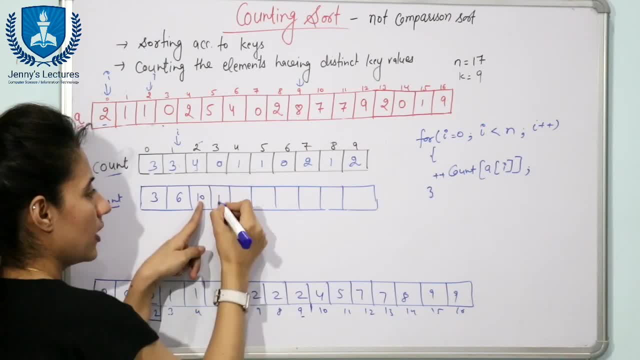 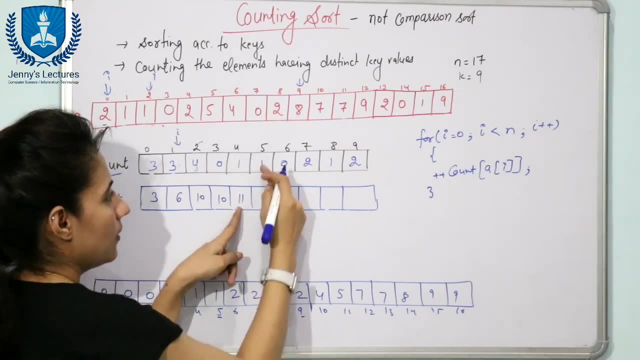 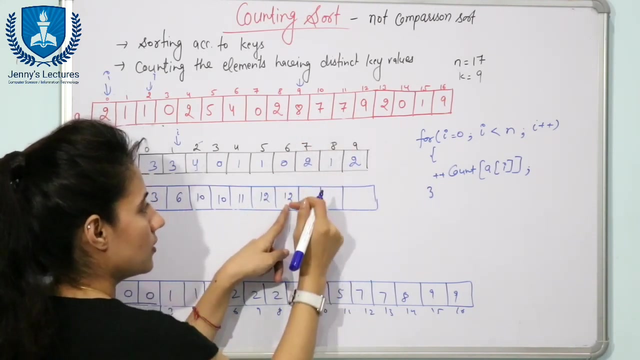 for this: 3, 10 plus 0, that is 10, only 10 plus this 1. this next element, that is 11, 10 plus 1, is 12. position for 6 is 12 plus 0, that is 12 for seven. for 7, that would be 12 plus 2, that is 14 for 8. 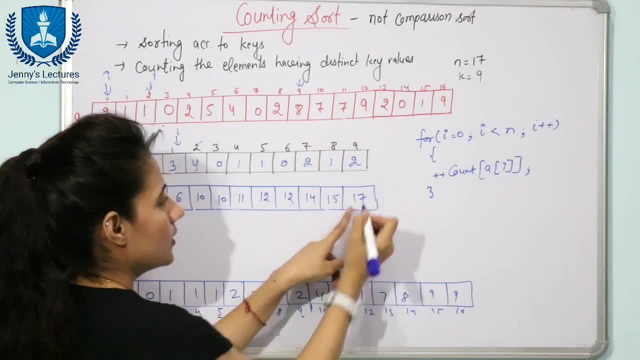 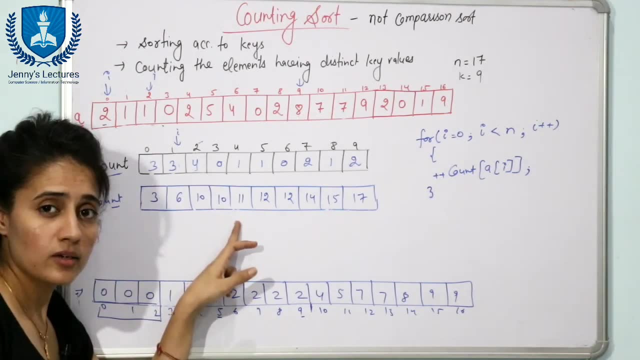 8, 14 plus 1, 15, 15 plus 2, 17 for 9 it is 17. so this is how now the updated count array. so now this array is going to reflect the actual position of this element in the sorted array now. 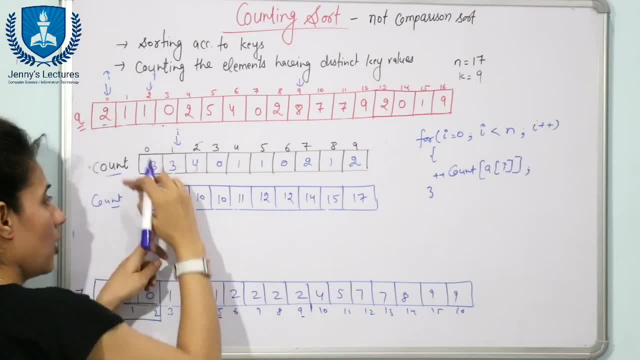 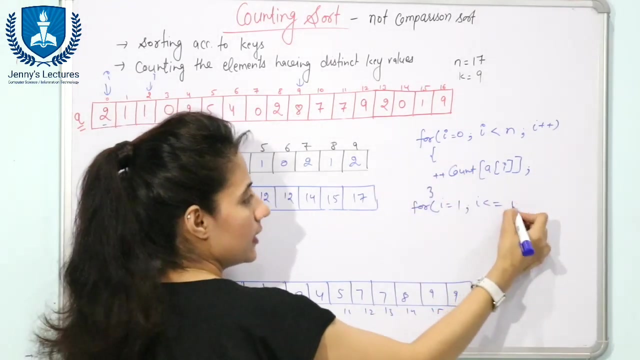 i am going to write down the code. fine, see how to update this count array. see, one for loop would be there. we are going to start the for loop from 1, so i is equal to 1. i less than equal to k. value k is 9, so i less than equal to 9 and i plus plus. 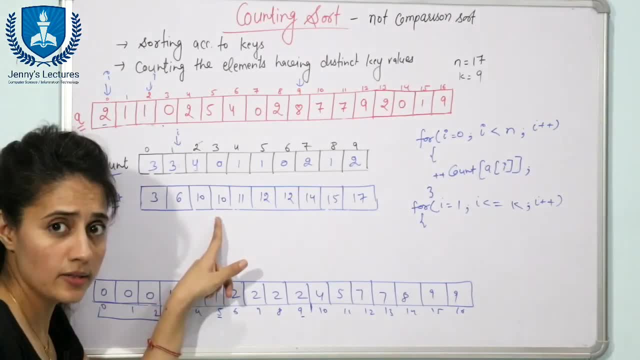 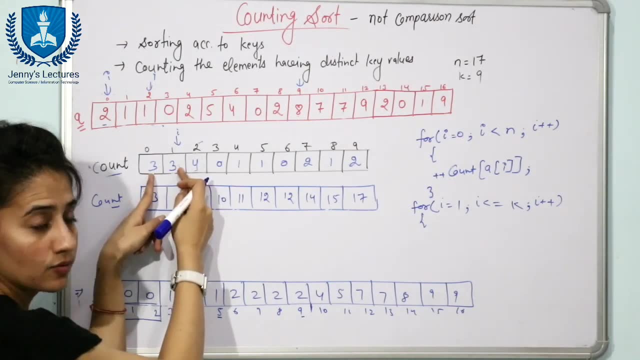 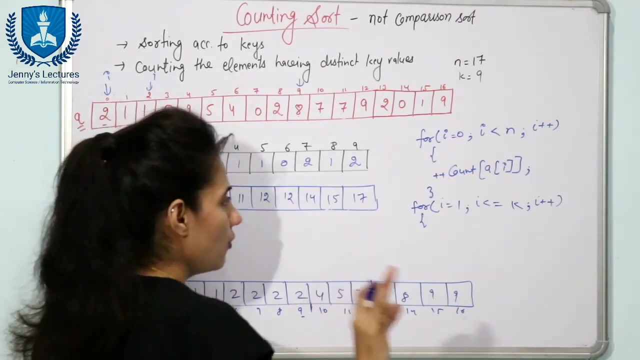 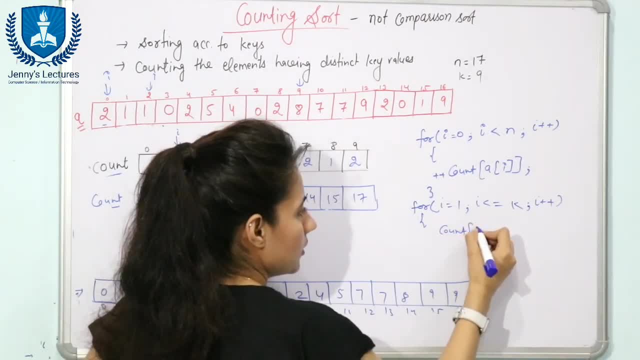 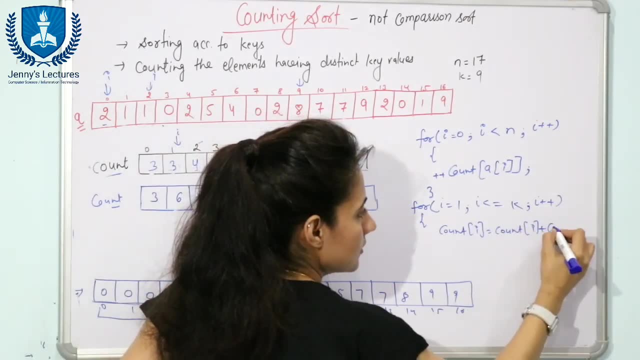 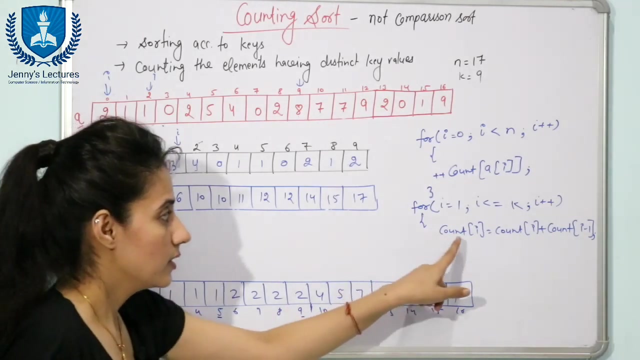 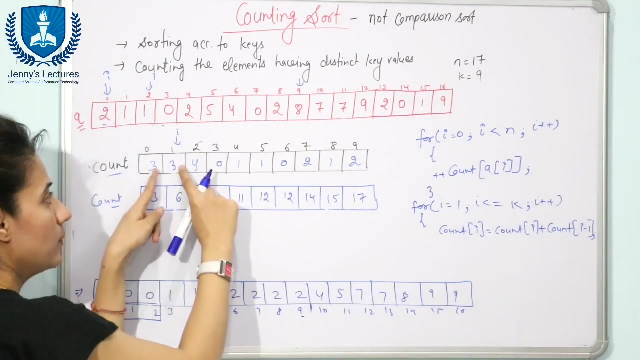 do this. see this count of i would be count of i plus count of i minus 1. see i, we have started from 1. that is why count 1 here count 1. this count 1 would be 3 plus 3, that is 6 means count of i plus previous value, i minus 1. sorry, 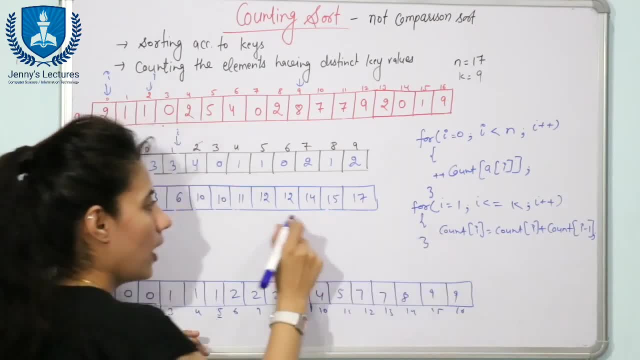 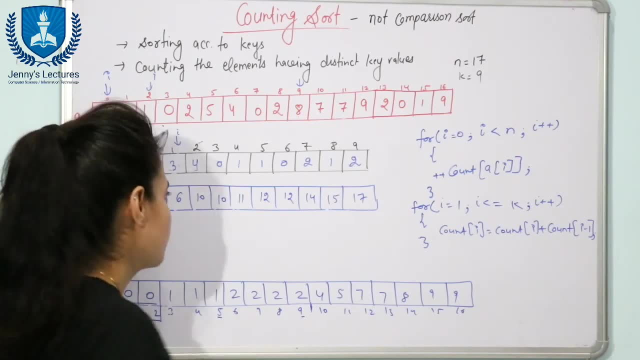 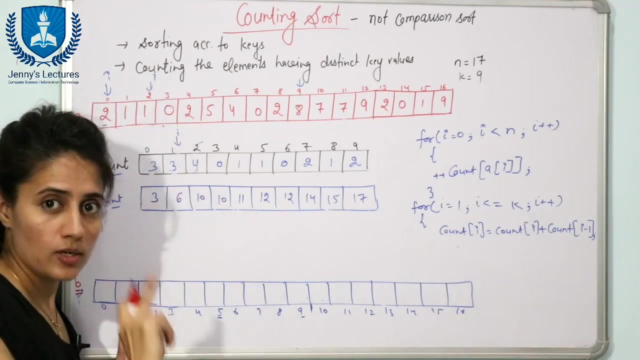 i minus 1. fine, so this is how we are going to update this array. now we are going to build the output array, how we are going to build this array, this output array. see, see, we have taken one another array. the name is suppose b, the size is same as the original array, having element 17. 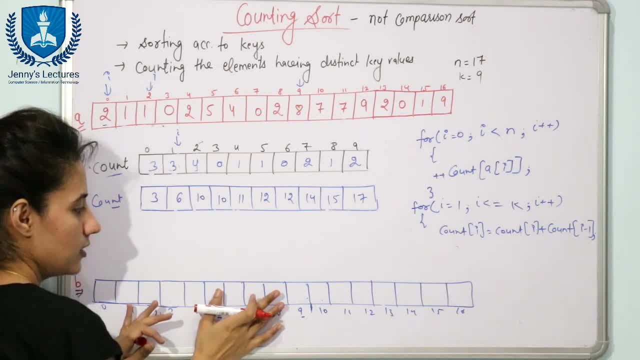 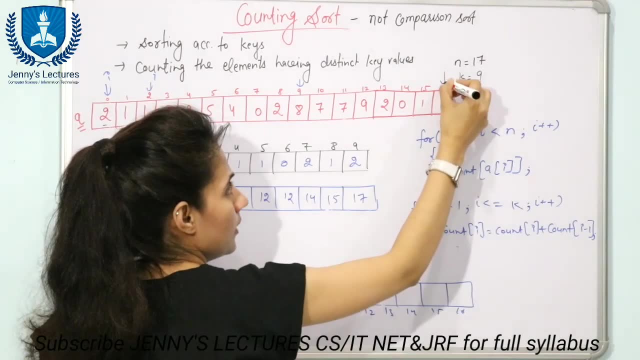 total element 17: how we are going to fill this array. this array would be sorted array. see, this is our original array. we are going to scan this array from right to left, from higher. this array are going to take one variable. why i am going to start from here. 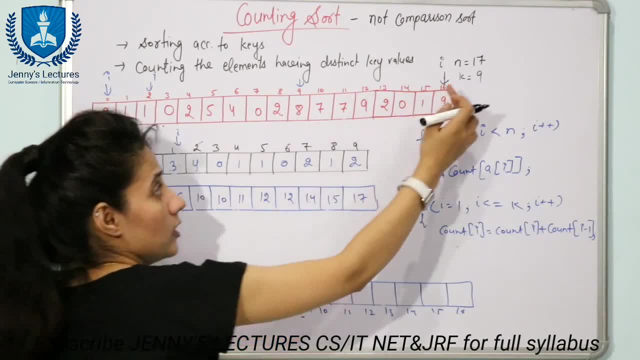 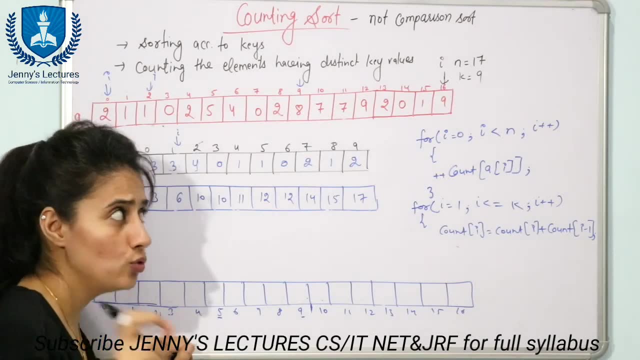 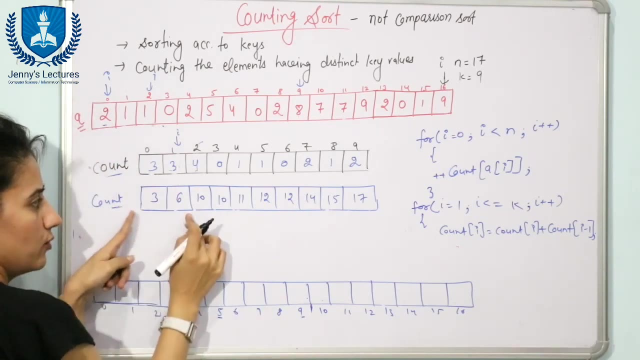 i am going to tell you that thing also. first of all, see, suppose i am going to start from here. the value is 9, key value is 9. so what you have to do in count, in count array, you, just you just go say this is our updated count array. we, we are going to see this array now. 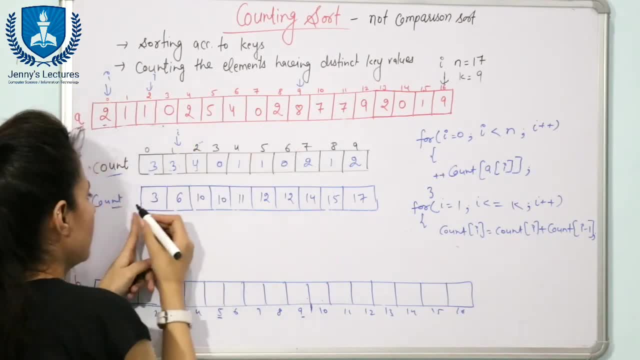 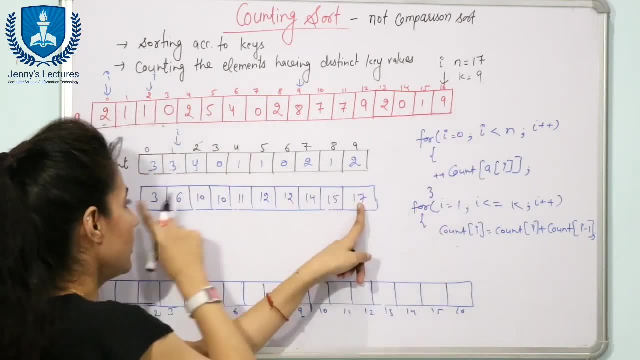 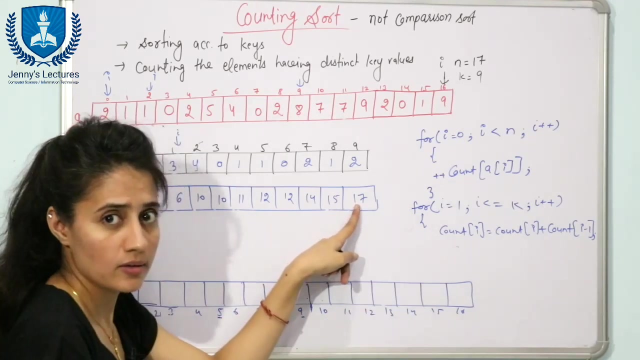 we are not going to see this one. so see, just go to the index 9. this is index 9. all it is right value is 9. go to index 9 in count array. right, but we cannot store 9 at 17 because we don't have 17. this is the count, but we are actually working on the index now. so first, 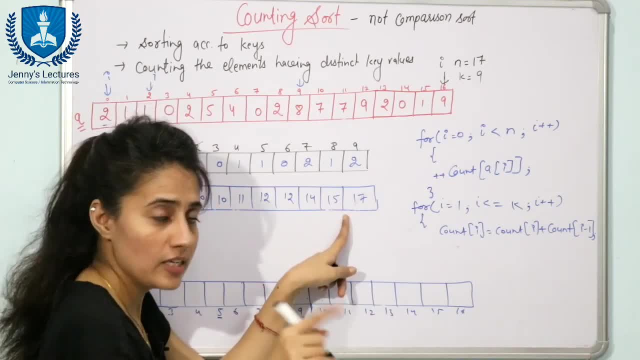 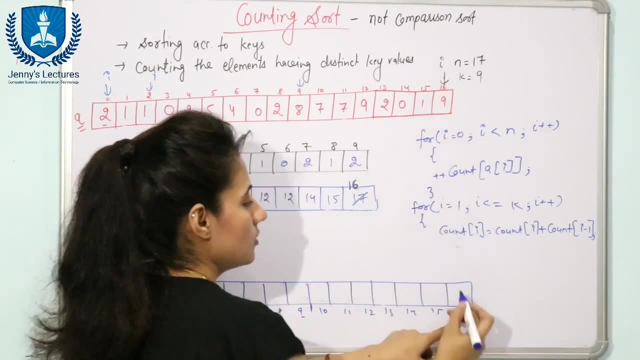 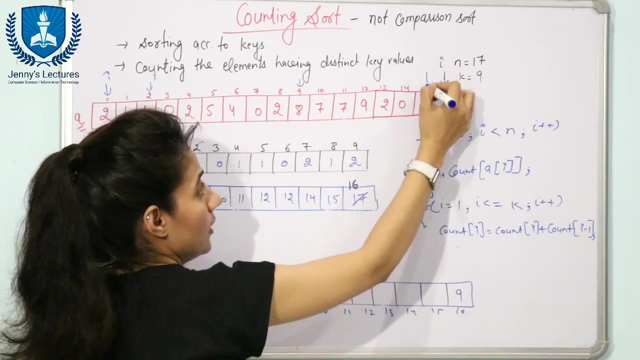 of all. we are going to decrement this by 1- 17 minus 1, that is 16, and in the output array go to the index 16 and store this 9. this is the actual place for this 9. fine, now decrement i. now i is at this place. find out the value at this, that is 1. now go to the index 1 in this. 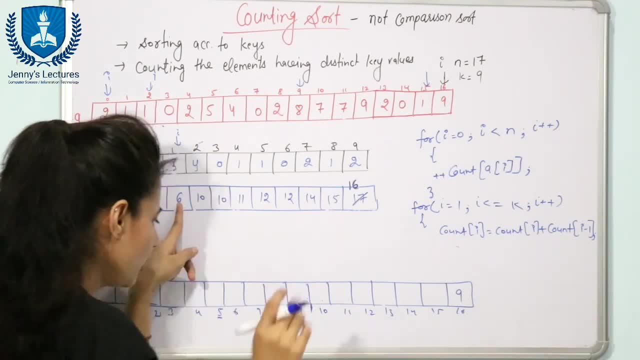 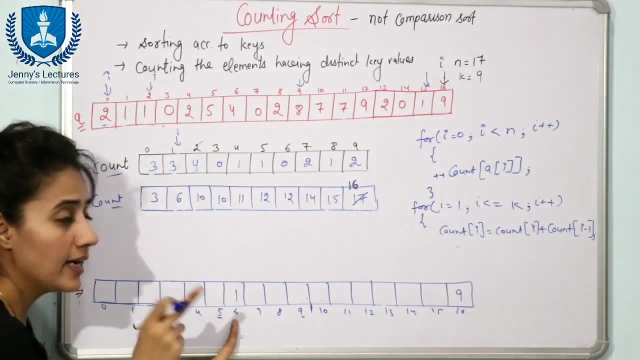 count array. index 1 value is 6, but we are not going to store 1 here. why so? because this is count value, but we are. we are going to store at index 5. fine, so first of all, we are going to store 1 here. so, first of all, we are going to store 1 here. so we are going to 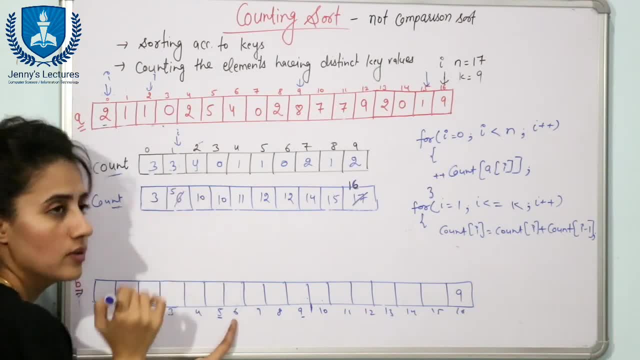 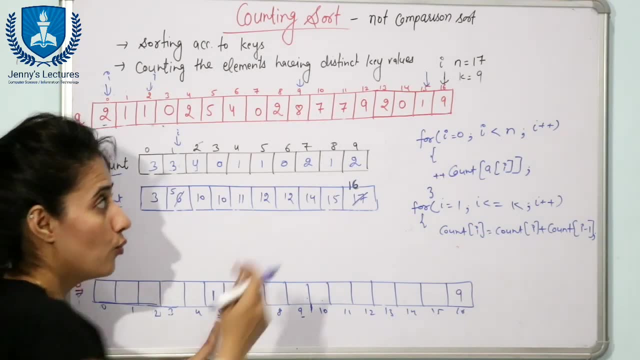 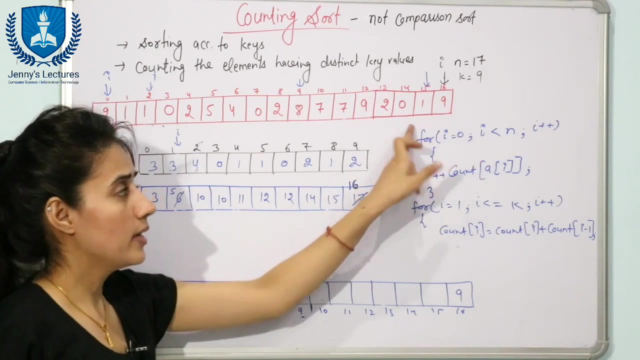 we are going to decrement this by 1, that is 5, and now we are going to store at 5. here we got 1. fine, why we have started from here? see, you can start from here, you will get sorted array, but i am going to start from here just to maintain the stability of this counting sort. now, what is? 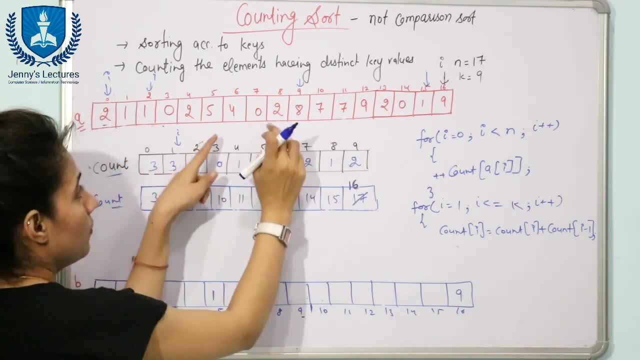 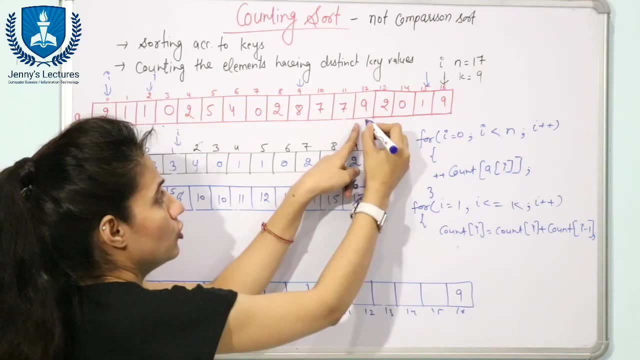 that stability of sort. see, let us suppose in this case, in this case this is 9 and this is 9. both are same, 9 and 9. the position of this is 12, index is 12 and index is 16. so this 9 is. 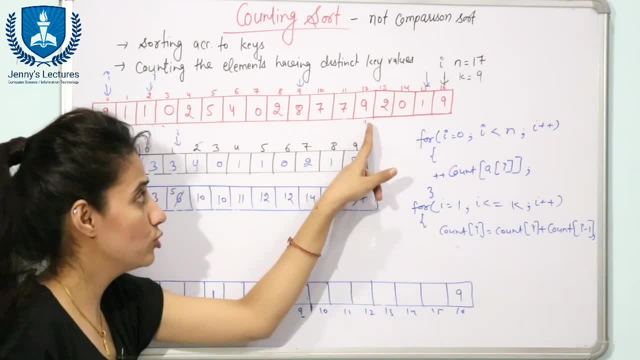 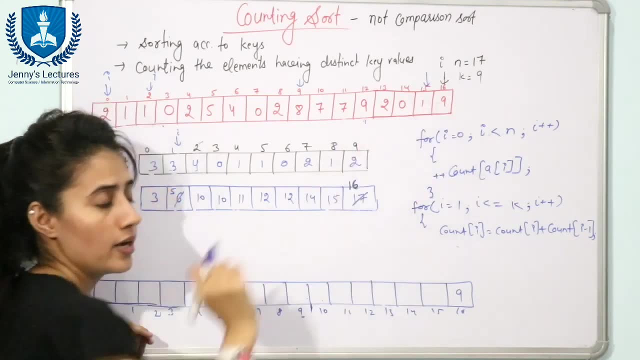 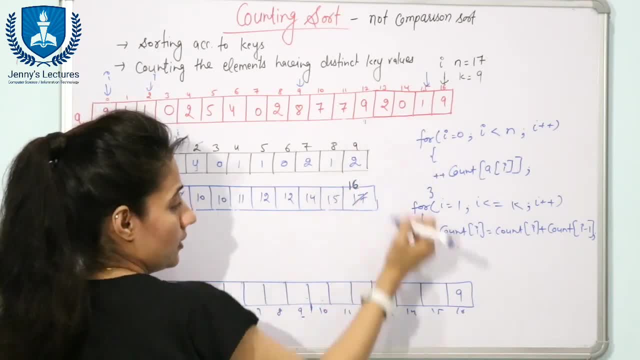 before this 9. that is the stability. before this 9, that is the stability, that is the stable sort. although we can, that is the stable sort. although we can, that is the stable sort. although we can write, write, write in the sorting, in the sorting, the sorted. 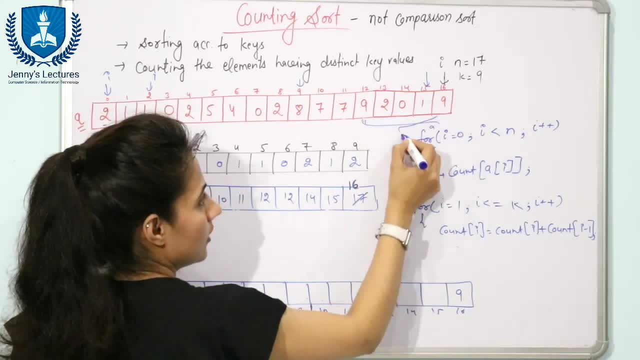 in the sorting, in the sorting, the sorted. in the sorting, in the sorting, the sorted array. you can write this 9 array. you can write this 9 array. you can write this 9 here and this 9 at this place. here and this 9 at this place. 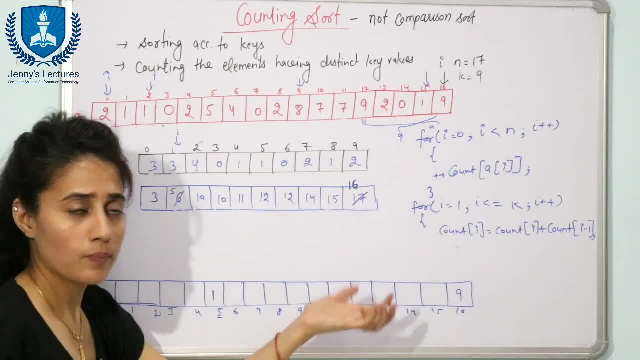 here and this 9 at this place, but the value is same. obviously the array, but the value is same. obviously the array, but the value is same. obviously the array would be sorted, but this will not would be sorted, but this will not. would be sorted, but this will not maintain the stability of the sorting. 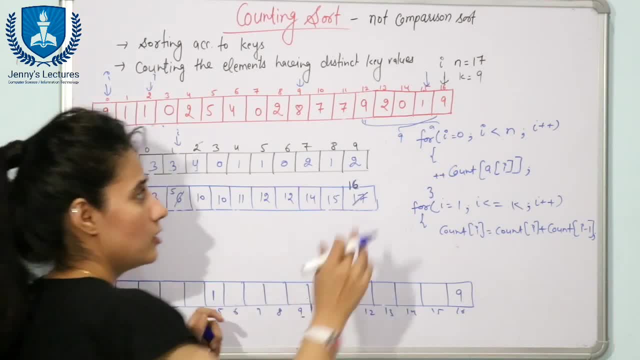 maintain the stability of the sorting, maintain the stability of the sorting algorithm. fine if you start from here, algorithm. fine if you start from here, algorithm fine if you start from here. only that is why. to maintain just the only, that is why to maintain just the only that is why to maintain just the stability. i'm going to start from. 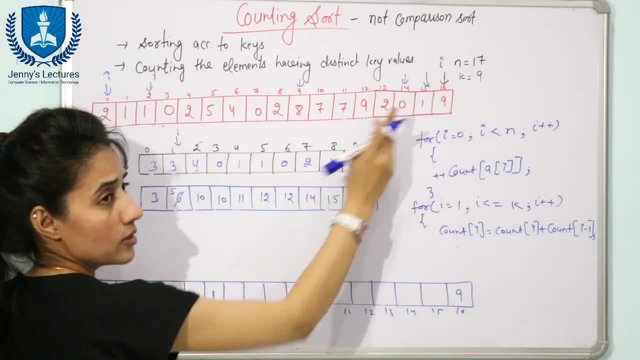 stability. i'm going to start from stability. i'm going to start from here now decrement i here, now decrement i here, now decrement i now here. value is zero. go to the index now here. value is zero. go to the index now here. value is zero. go to the index zero. value is three. first decrement: this: 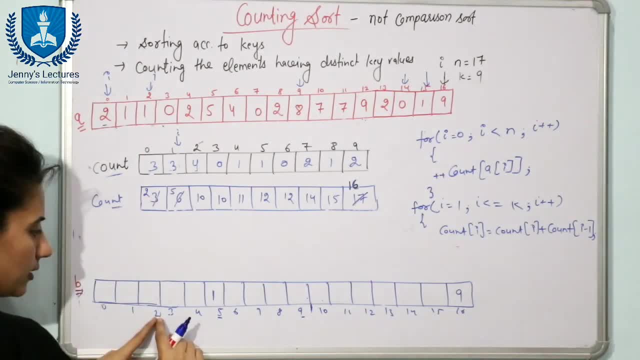 zero value is three first decrement. this zero value is three first decrement. this value, that is two now in this output value. that is two now in this output value. that is two now in this output array at index. two store array at index. two store array at index. two store zero. 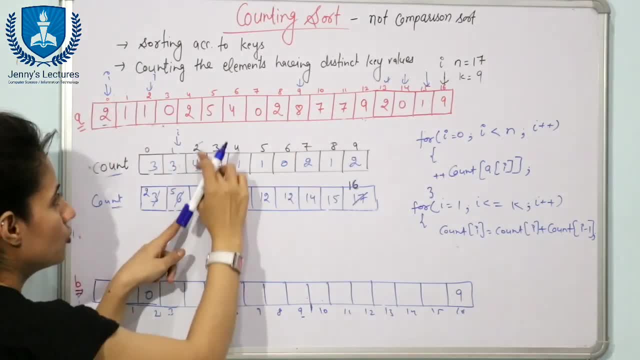 zero, zero. next decrement: i value is two. go to the next decrement: i value is two. go to the next decrement: i value is two. go to the index two value is ten. index two value is ten. index two value is ten. but first of all, decrement this, that is: 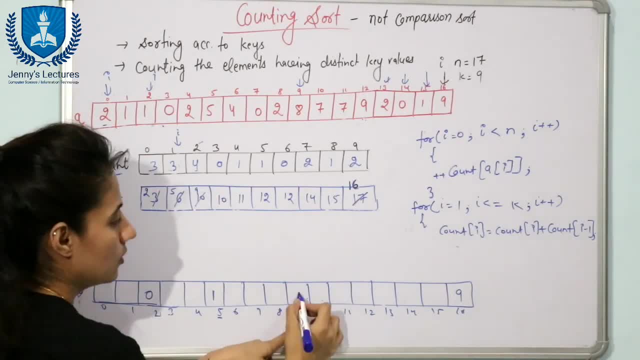 but first of all decrement this, that is, but first of all decrement this. that is nine. and now at ninth index store nine. and now at ninth index store. nine. and now at ninth index store. what, what, what? two, now again: decrement value is nine now. two, now again. decrement value is nine now. 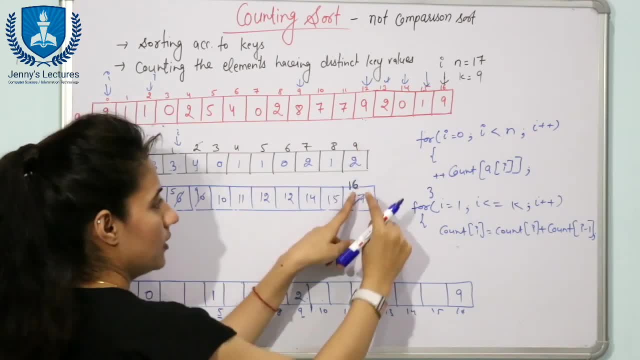 two. now again, decrement value is nine. now see, see, see again. go to the index 9 at index 9, again. go to the index 9 at index 9, again go to the index 9 at index 9. updated value is 16. but first of all we. 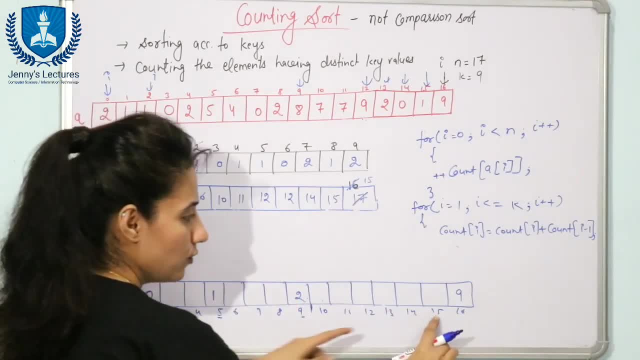 updated value is 16, but first of all, we updated value is 16, but first of all we are going to decrement this, that is 15, are going to decrement this, that is 15, are going to decrement this, that is 15. and at 15th index in output array, you 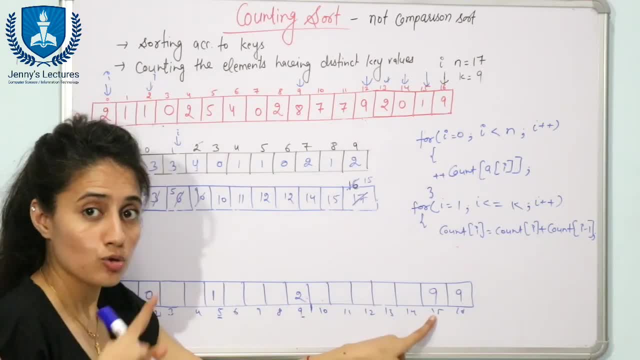 and at 15th index in output array, you and at 15th index in output array, you are going to store this, are going to store this, are going to store this. nine: so see as you can see here. nine, so see as you can see here. 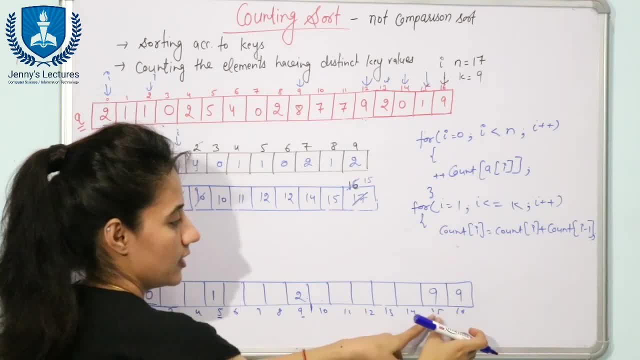 nine. so see, as you can see here, this, this nine is at place 15th and this, this nine is at place 15th and this, this nine is at place 15th and this nine is at 16 and 15 is. this nine is at 16 and 15 is. 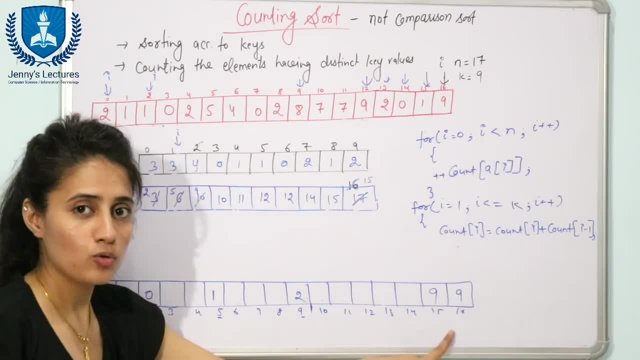 this nine is at 16 and 15 is before 16. or you can say less than 16 before 16, or you can say less than 16 before 16, or you can say less than 16. so this is how we are going to maintain. 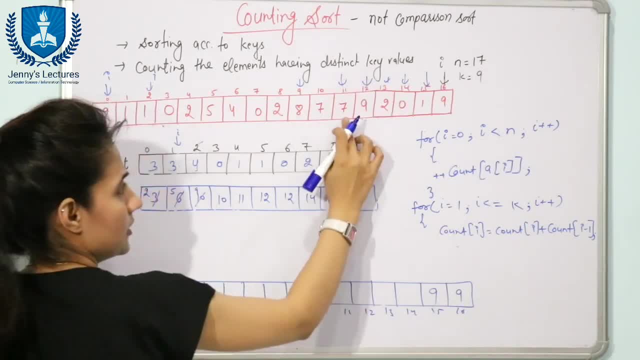 so this is how we are going to maintain. so this is how we are going to maintain the stability fine, the stability fine, the stability fine. now decrement again i 7. now decrement again: i 7. now decrement again, i 7. now go to the index 7. here is 7 in the 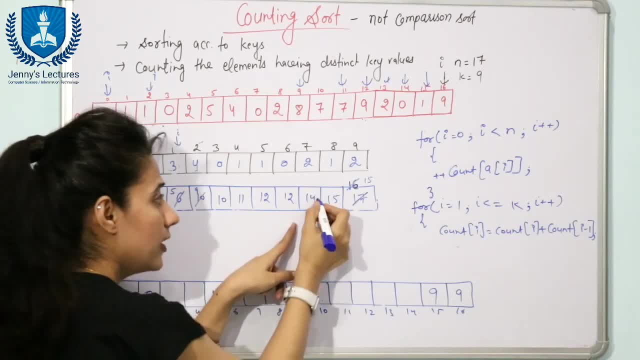 now go to the index 7. here is 7 in the. now go to the index 7. here is 7 in. the updated count sort value is 14. updated count sort value is 14. updated count sort value is 14. first of all decrement this, that is 13. 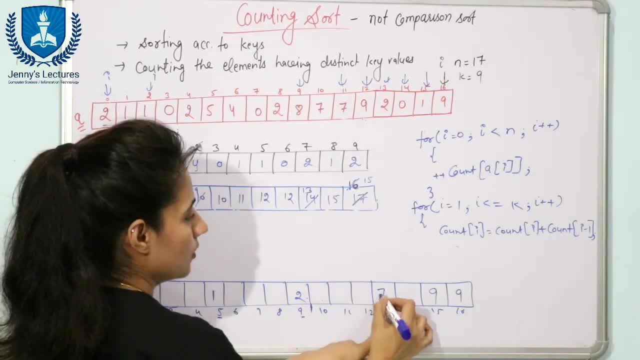 first of all, decrement this, that is 13. first of all decrement this, that is 13. and at the index 13, now store, and at the index 13, now store. and at the index 13, now store. 7 again decrement i value we have. 7 again decrement i value, we have. 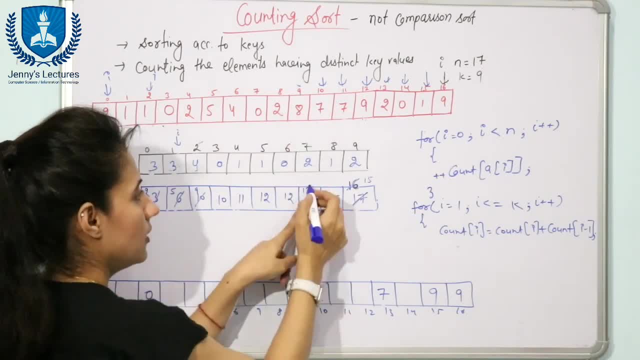 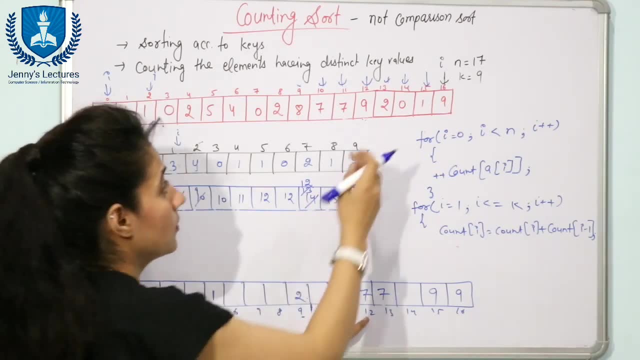 7. again decrement i value. we have again 7. go to the index 7. value is 13, again 7. go to the index 7. value is 13, again 7. go to the index 7. value is 13. store 7. decrement this, that is 8. 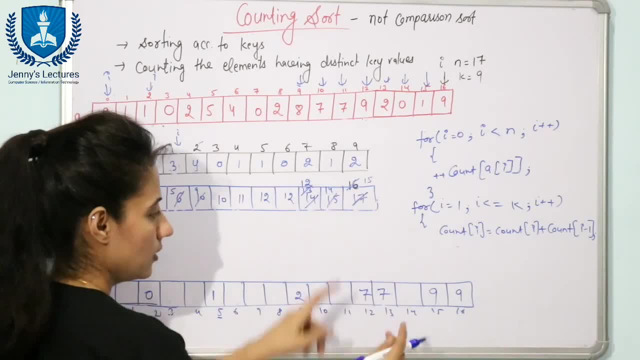 store 7, decrement this: that is 8. store 7, decrement this: that is 8. go to the index 8 value is 15 decrement. go to the index 8 value is 15 decrement. go to the index 8 value is 15 decrement this: that is 14. at 14th, store 8. 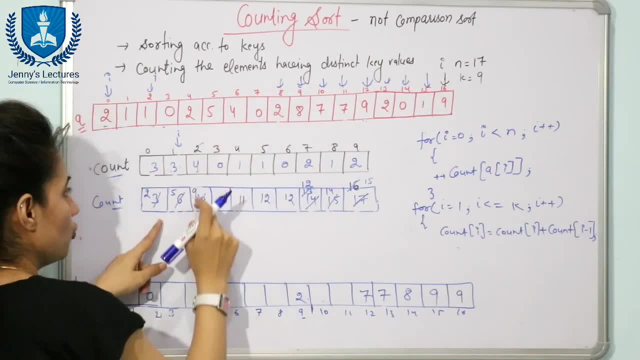 this, that is 14 at 14th, store 8. this, that is 14 at 14th, store 8. decrement this, so the value is 2. now go decrement this, so the value is 2. now go decrement this, so the value is 2. now go to the index 2 in this count array. 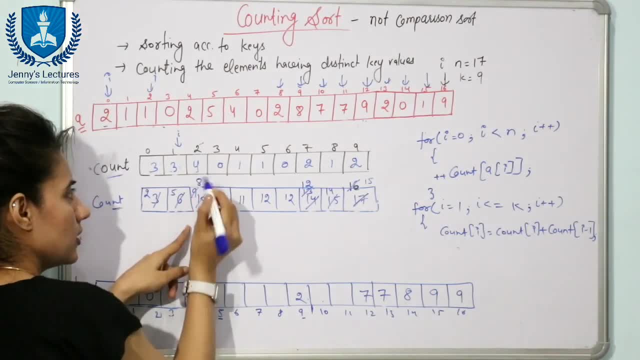 to the index 2 in this count array. to the index 2 in this count array. at index 2, value is 9, first decrement at index 2. value is 9, first decrement at index 2. value is 9, first decrement. this value, that is. 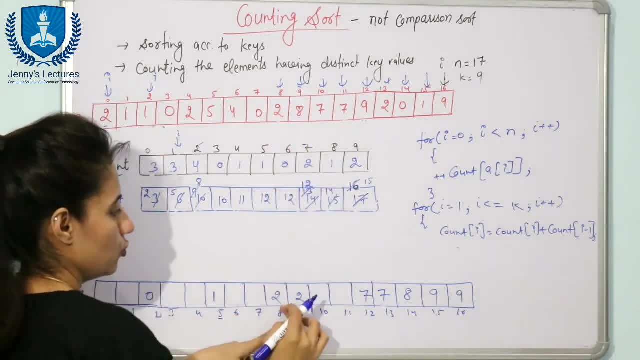 this value, that is this value. that is 8 at 8th index. now we are going to store 8 at 8th index. now we are going to store 8 at 8th index. now we are going to store this value, this value. 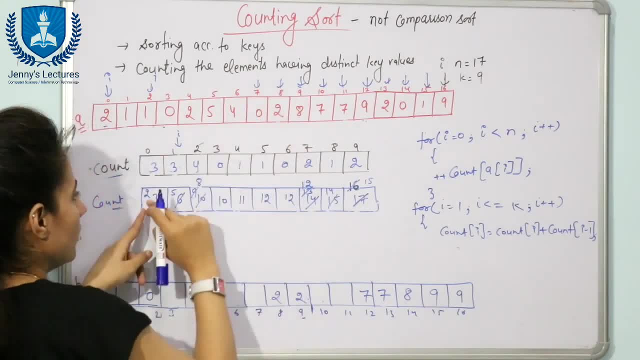 this value: 2 decrement this: i value now 0. go to the 2 decrement this: i value now 0. go to the 2 decrement this: i value now 0. go to the index 0 value is 2 decrement this. index 0 value is 2 decrement this. 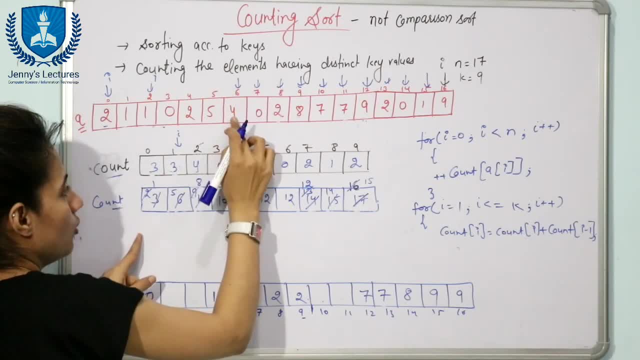 index 0 value is 2, decrement this: 1. we are going to store 0 here, decrement 1. we are going to store 0 here, decrement 1. we are going to store 0 here, decrement this one value is 4. go to the index 4. 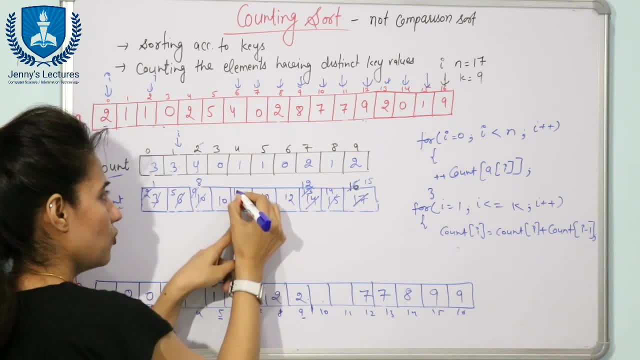 this one value is 4. go to the index 4. this one value is 4. go to the index 4. here the value is 11 decrement this first. here the value is 11 decrement this first. here the value is 11 decrement this first of all. 10. at 10th index we are going. 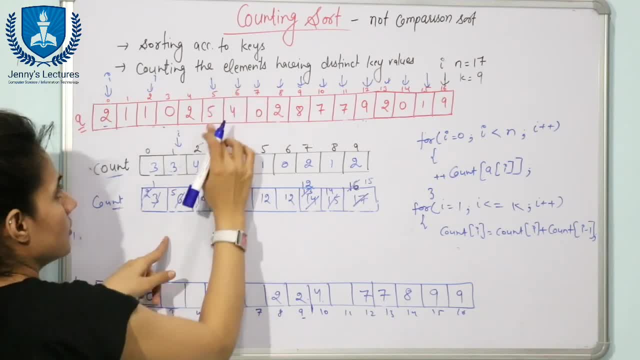 of all 10 at 10th index. we are going of all 10 at 10th index. we are going to store, to store. to store 4. now determine this here. the element is 4. now determine this here. the element is 4. now determine this here. the element is 5. key value is 5. go to the index 5. 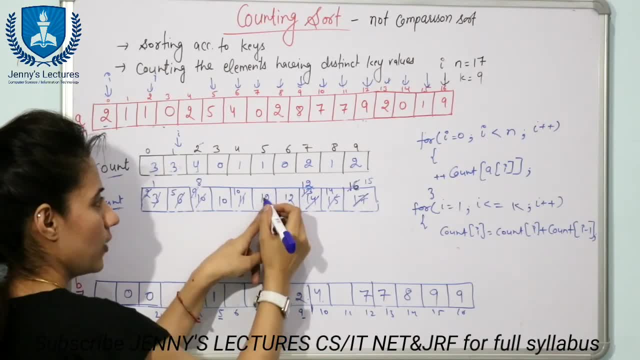 5. key value is 5. go to the index 5: 5. key value is 5. go to the index 5. at index 5. in the count array here: the. at index 5. in the count array here: the at index 5. in the count array here, the value is: number is 12. 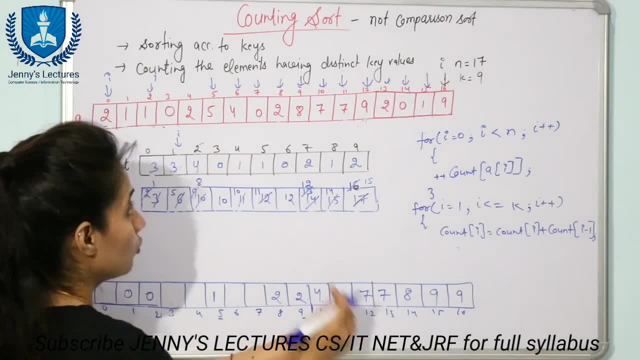 value is number is 12. value is number is 12 decrement. this, first of all, that is 11 decrement. this, first of all, that is 11 decrement. this, first of all, that is 11 at 11, we are going to store now. at 11, we are going to store now. 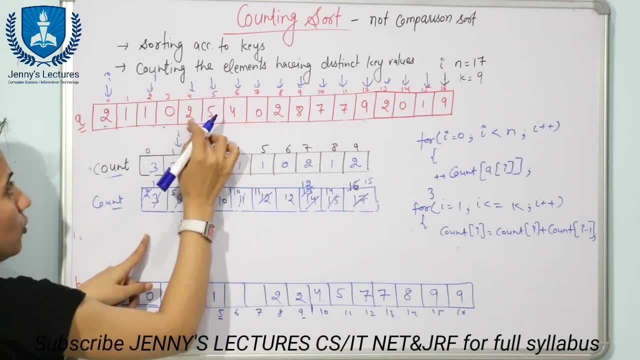 at 11. we are going to store now 5. fine again decrement. i value now 5. fine again decrement. i value now 5. fine again decrement. i value now. here the key value is 2. go to the index. here the key value is 2. go to the index. 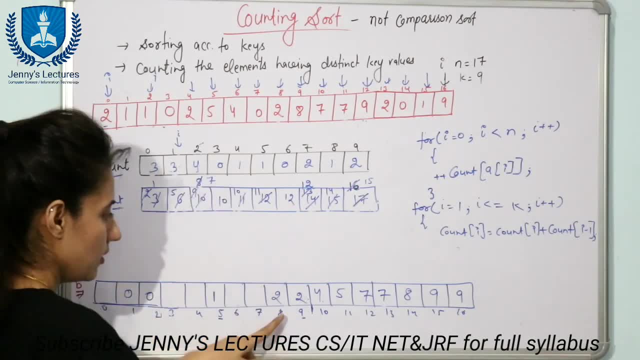 here the key value is 2. go to the index: 2. here the value is 8, decrement this 2. here the value is 8 decrement this 2. here the value is 8 decrement this. first of all, seven, now at seven we are. first of all seven, now at seven, we are. 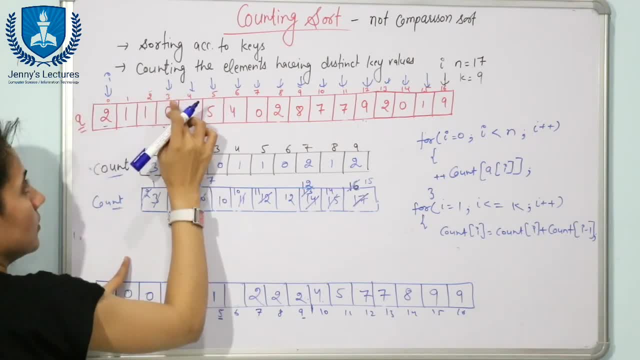 first of all, seven. now at seven, we are going to store two. going to store two. going to store two now. go to this. this place value is now. go to this. this place value is now. go to this. this place value is zero. go to the index: zero. here we have one. 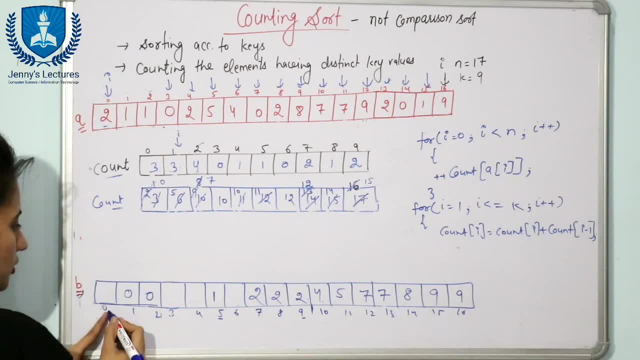 zero. go to the index zero. here we have one zero. go to the index zero. here we have one decrement: this, that is zero. decrement this, that is zero. at this, at the zeroth index. we are going at this at the zeroth index. we are going at this, at the zeroth index. we are going to store. 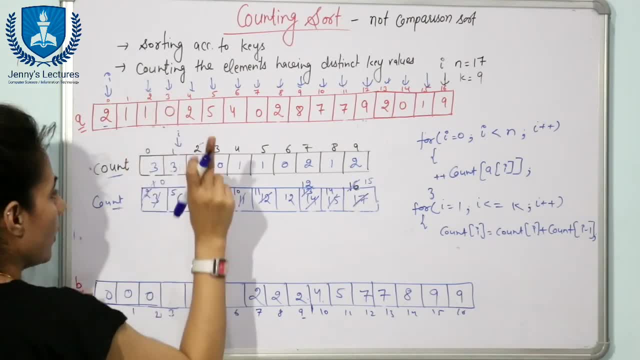 to store, to store: zero again decrement. i value here the zero again decrement. i value here the zero again decrement. i value here: the key value is one. key value is one. key value is one: go to the index. one value is five. go to the index. one value is five. 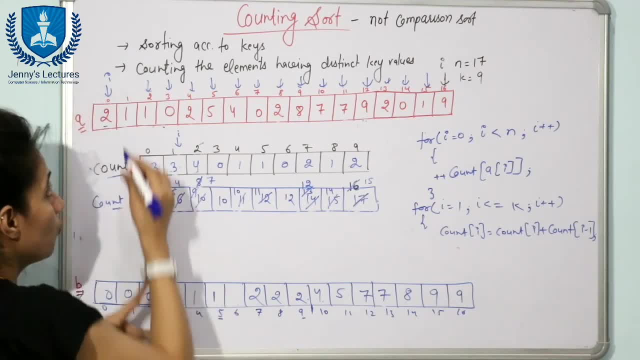 go to the index. one value is five. decrement this, first of all four. decrement this, first of all four. decrement this, first of all. four at four, we are. we are going to store one at four, we are. we are going to store one at four, we are. we are going to store one again. decrement one: 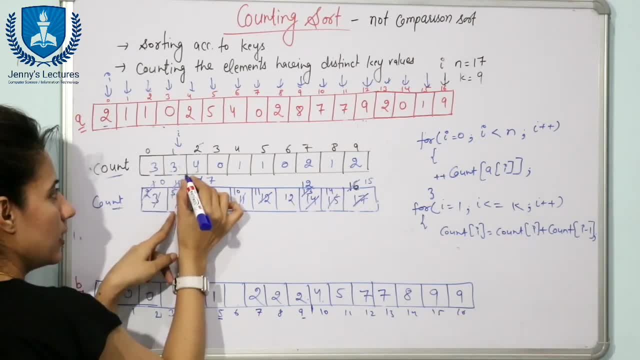 again decrement one. again decrement one. go to this index. one value is four: go to this index. one value is four. go to this index. one value is four, decrement this: that is three at third. decrement this: that is three at third. decrement this: that is three at third. we are going to store one. 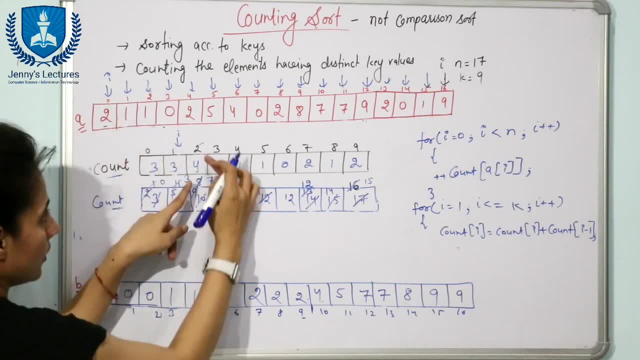 we are going to store one. we are going to store one. now. decrement this two. now now decrement this two. now now decrement this two. now at index two. value is seven: see updated at index two. value is seven: see updated at index two. value is seven: see updated value is seven. we are going to decrement. 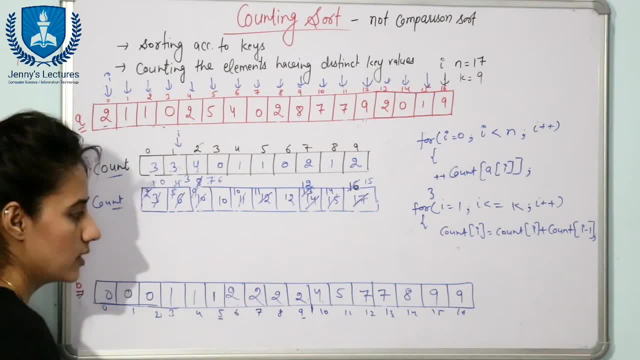 value is seven. we are going to decrement value is seven. we are going to decrement this. that is this. that is this. that is six at sixth. we are going to place this six at sixth. we are going to place this six at sixth. we are going to place this two. now fine, and we are going to stop. 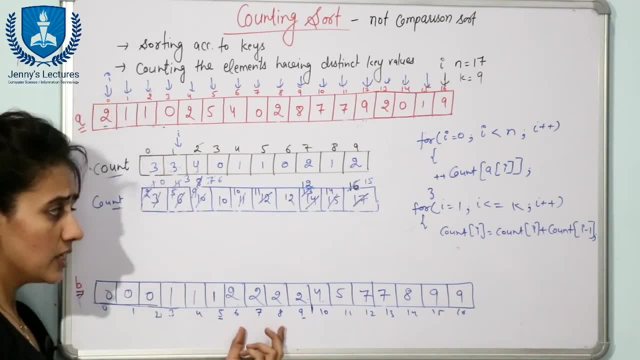 two now, fine, and we are going to stop. two now, fine, and we are going to stop. because we have reached to zeroth index, because we have reached to zeroth index, because we have reached to zeroth index now you can say: this is the sorted array. 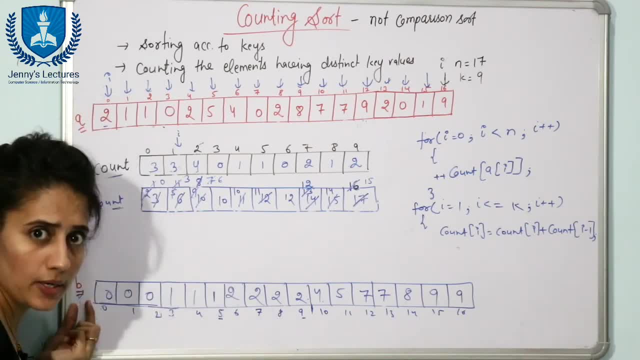 now you can say: this is the sorted array. now you can say: this is the sorted array, fine, so we have taken another array. that fine, so we have taken another array. that fine, so we have taken another array. that is b now, simply what you have, you will. 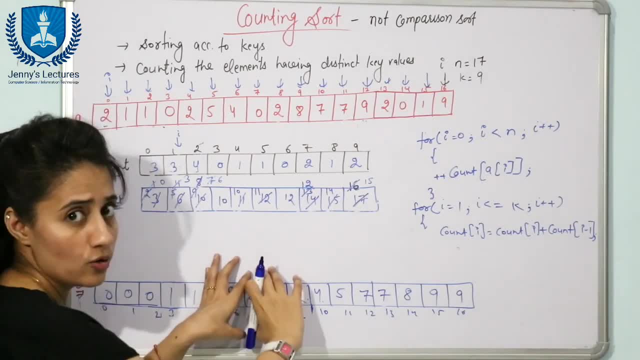 is b now simply what you have you will? is b now simply what you have you will? do you simply copy the content of this? do you simply copy the content of this? do you simply copy the content of this array, the element of this array to array? the element of this array to. 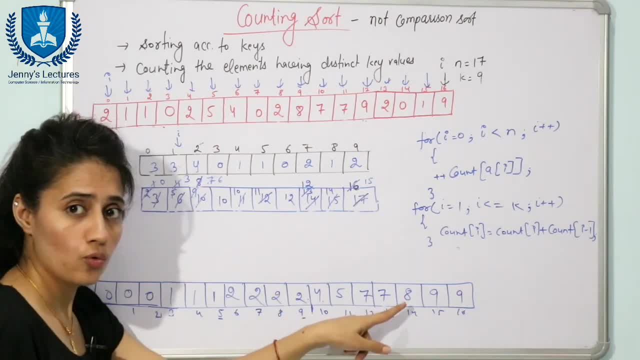 array, the element of this array, to this array with a for loop now. how to this array with a for loop now. how to this array with a for loop now? how to write down this thing into code. how to write down this thing into code. how to write down this thing into code. how to build this array. see, we have just. 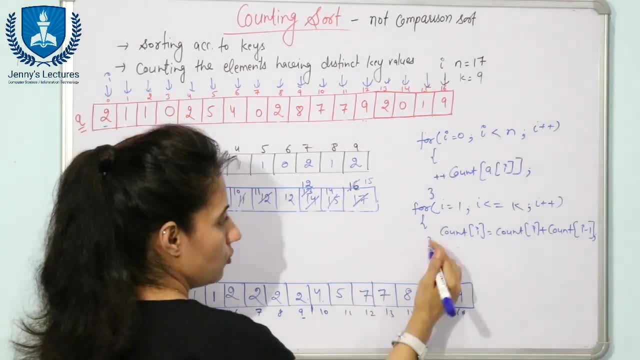 build this array. see, we have just build this array. see, we have just. this is one for loop for this. this is for. this is one for loop for this. this is for. this is one for loop for this. this is for loop for this: updated count and now. 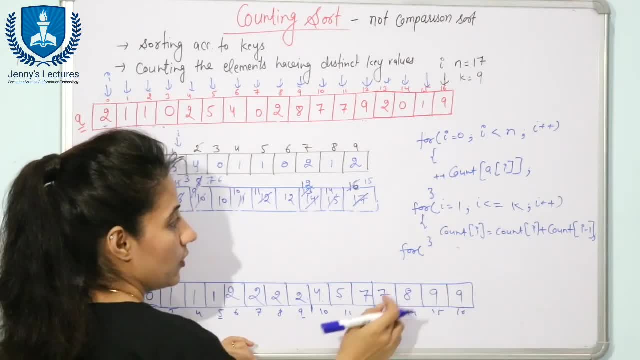 loop for this updated count and now loop for this updated count. and now this for loop is for this for loop is for this for loop is for building this output array. fine, we have building this output array. fine, we have building this output array. fine, we have started our for loop from here, fine, 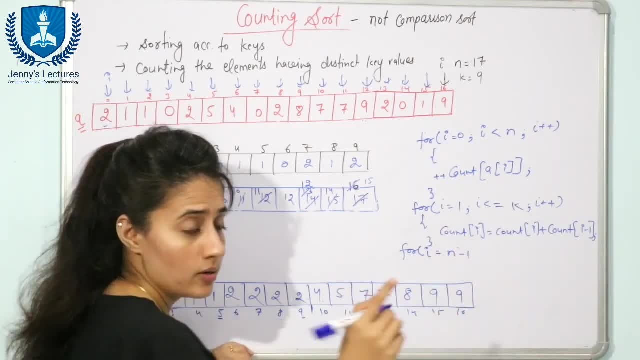 started our for loop from here, fine. started our for loop from here, fine. so i value would be. so i value would be. so i value would be: n minus 1. n minus 1. n minus 1 till i greater than equal to zero. till i greater than equal to zero. 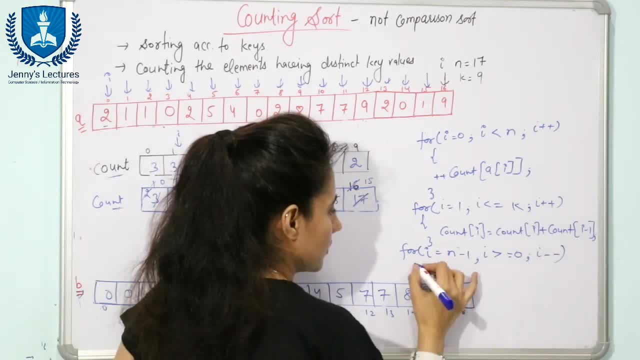 till i greater than equal to zero and i minus minus fine and i minus minus fine and i minus minus fine. now, within this for loop, what you will now within this for loop, what you will now within this for loop, what you will write, write, write, see, see. 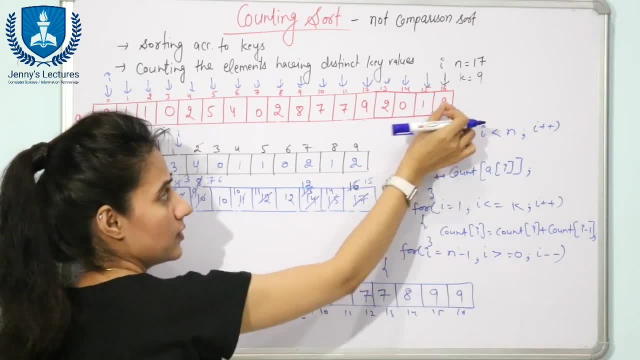 see, first of all, what we have done. first of all what we have done. first of all what we have done, we are going to take this value and you, we are going to take this value and you, we are going to take this value and you are going to place this value in the 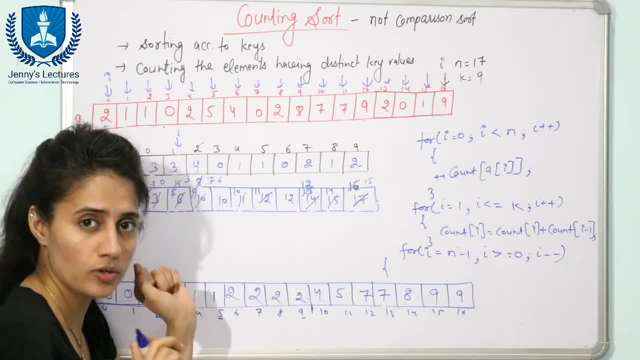 are going to place this value in the are going to place this value in the sorted array, after finding proper sorted array, after finding proper sorted array, after finding proper position, using this count position, using this count position, using this count array, fine, array, fine, array, fine. so take this value. 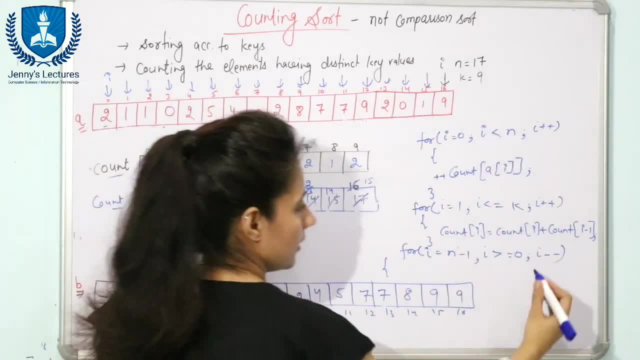 so take this value. so take this value, this value. how to take this value array, this value. how to take this value array, this value, how to take this value array. name is a and a of. i see a of. name is a and a of. i see a of. 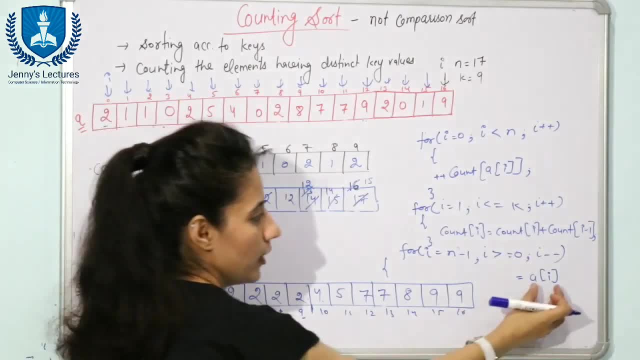 name is a and a of. i see a of i. this is how we are going to access i. this is how we are going to access i. this is how we are going to access this element. now where to put this? this element: now where to put this. 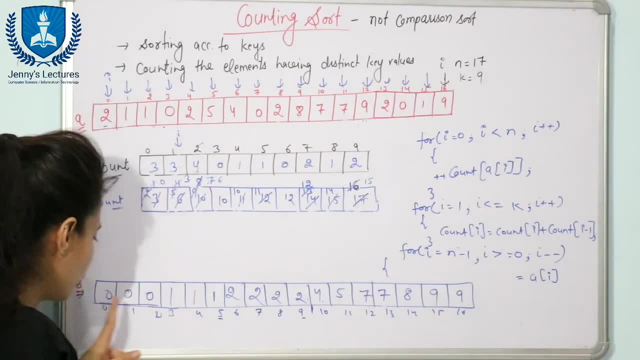 this element now, where to put this element to this side. what you will write. element to this side. what you will write. element to this side. what you will write. we are going to put this element in array. we are going to put this element in array. we are going to put this element in array b. but first of all you have to find out. 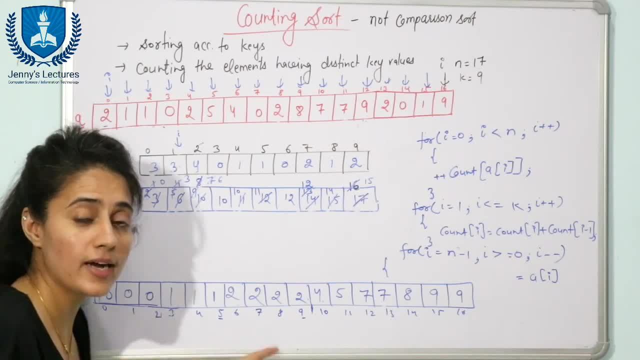 b, but first of all you have to find out b. but first of all you have to find out the proper index, the proper index, the proper index in this b for that index. what you will do in this b for that index, what you will do in this b for that index, what you will do, you will use count array. 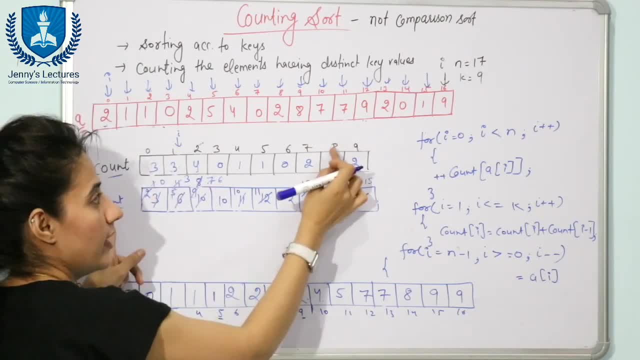 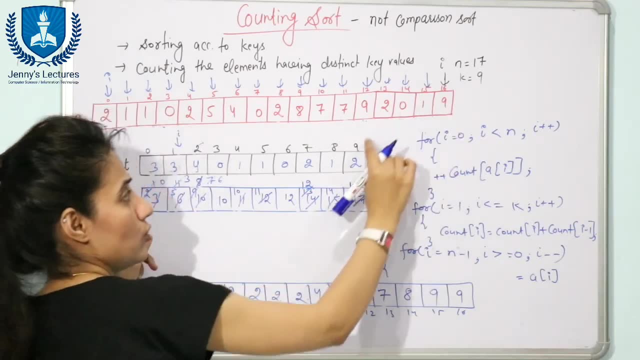 you will use count array. you will use count array fine and in count array also for finding fine and in count array also for finding fine and in count array also for finding this index, this index, this index. you will use this value. you will use this value. you will use this value. right, see, the value is 9, so same we are. 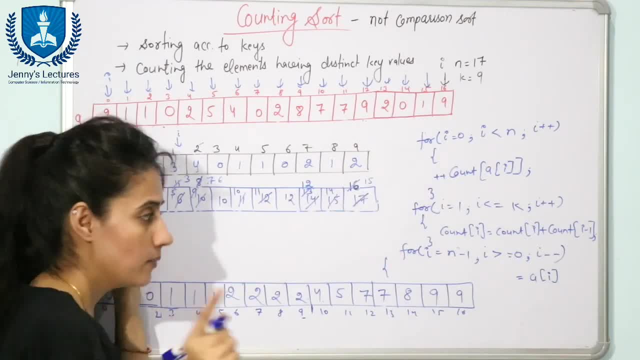 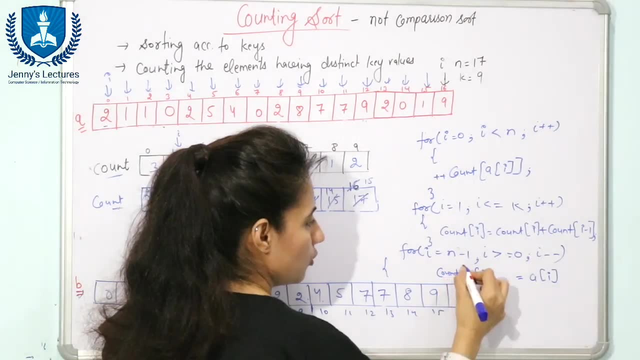 right, see, the value is 9, so same we are right, see, the value is 9, so same we are going to index 9. going to index 9, going to index 9, fine, see, so this is how we are going to right, right, right, count a of i. 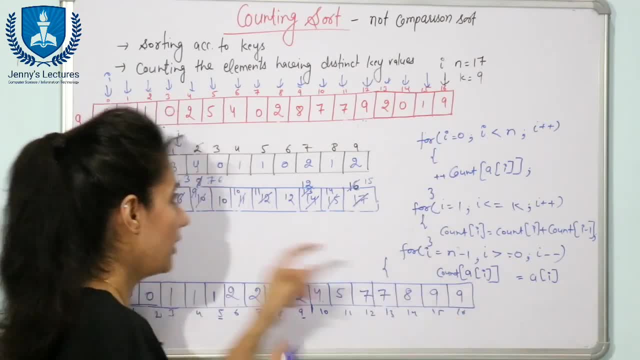 count a of i. count a of i, fine, see. let us suppose a of i is 9, so fine, see. let us suppose a of i is 9, so fine, see. let us suppose a of i is 9, so count 9. count of 9, this index. 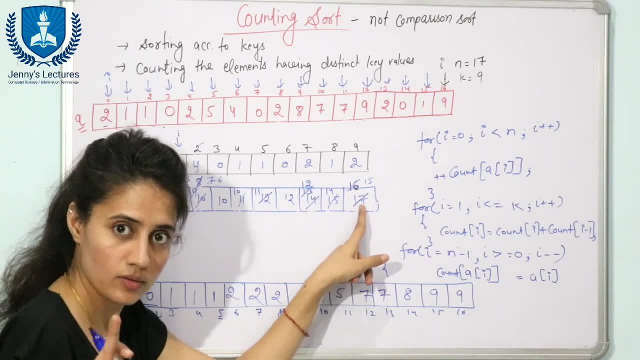 count 9, count of 9. this index: count 9, count of 9, this index. now what we have done: decrement this. now what we have done. decrement this. now what we have done. decrement this index, first of all index, first of all index, first of all. fine, so we will decrement this minus. 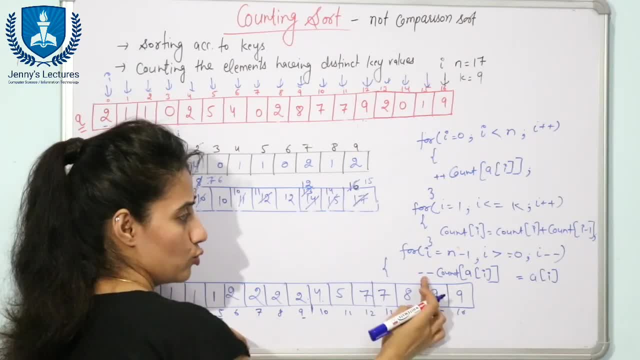 fine, so we will decrement this, minus. fine, so we will decrement this: minus, minus, minus, minus. see: first we will decrement, then we are see, first we will decrement, then we are: see, first we will decrement, then we are going to store, so pre-decrement, going to store, so pre-decrement. 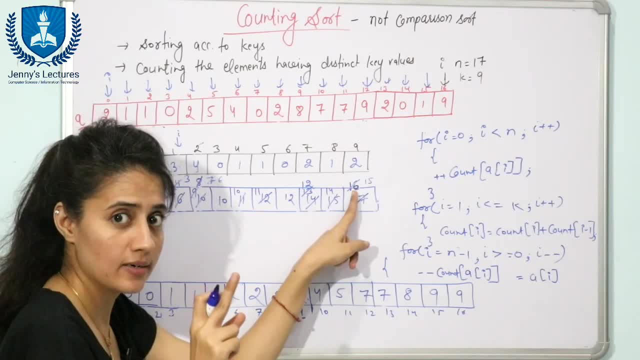 going to store. so pre-decrement. so after decrementing the value is what? so after decrementing the value is what? so? after decrementing the value is what? we have got 16, we have got 16. we have got 16. fine, now this 16 is the index. 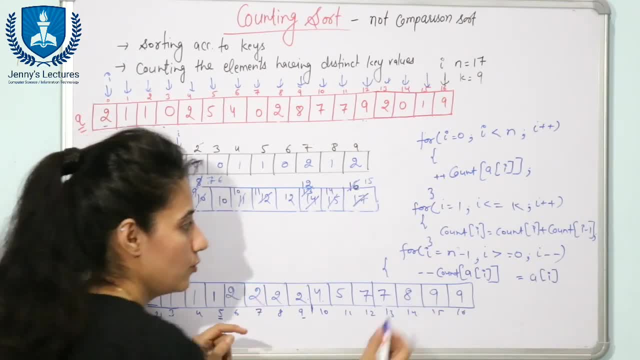 fine, now this 16 is the index. fine, now this 16 is the index in this area b, where we are going to in this area b, where we are going to in this area b, where we are going to store this value. store this value, store this value, fine, so this is. 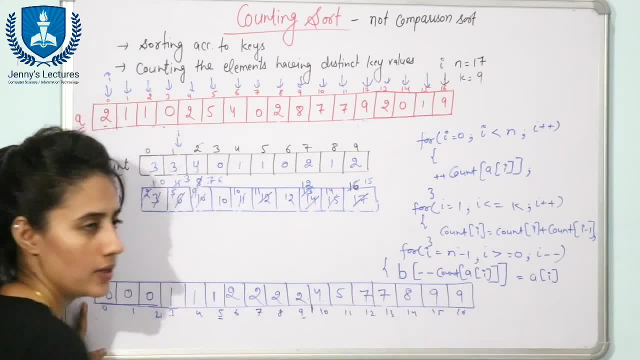 fine, so this is fine. so this is the index and name is the index and name is the index and name is array array, array b, b, b. so in b array, this is the index you are, so in b array, this is the index you are, so in b array, this is the index you are going to calculate. 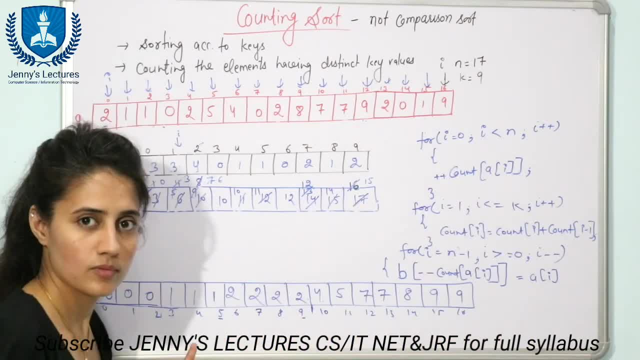 going to calculate, going to calculate where you are going to store the value, where you are going to store the value, where you are going to store the value a of i, a of i, a of i, fine, fine, fine, this is how we are going to build this. 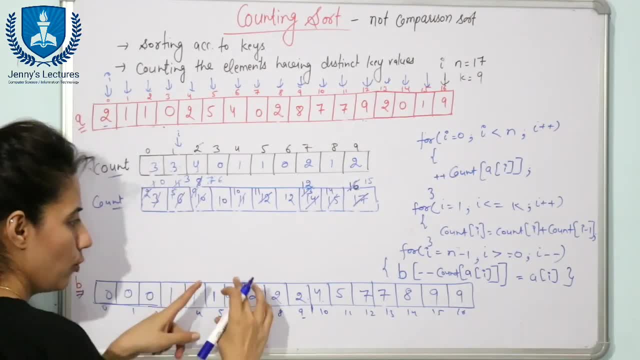 this is how we are going to build this. this is how we are going to build this array. so now, at last, one another for array. so now, at last, one another for array. so now, at last, one another for loop. would be there just to copy the loop. would be there just to copy the. 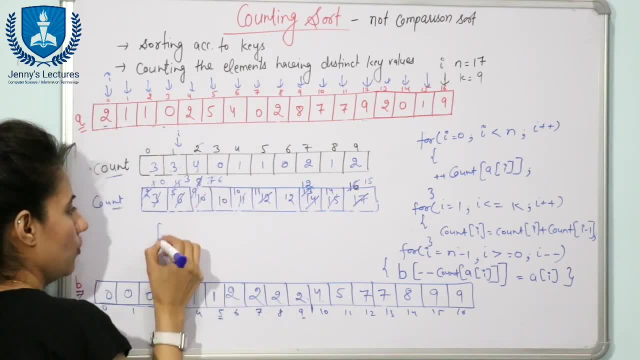 loop would be there just to copy the value of this array into value of this array, into value of this array into the original array. so what you can write the original array, so what you can write the original array, so what you can write after this: for loop for i is equal to. 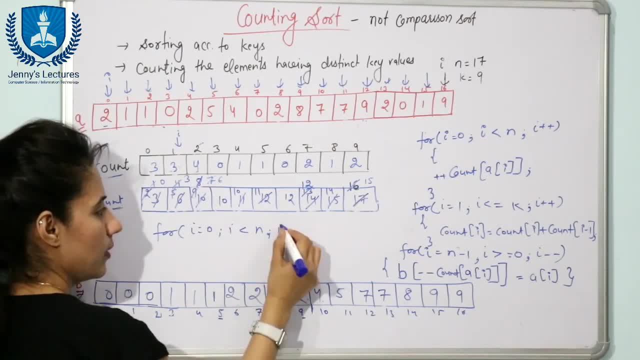 after this for loop for i is equal to. after this for loop for i is equal to zero, to i is equal to less than n. or zero to i is equal to less than n. or zero to i is equal to less than n. or less than equal to n minus one. 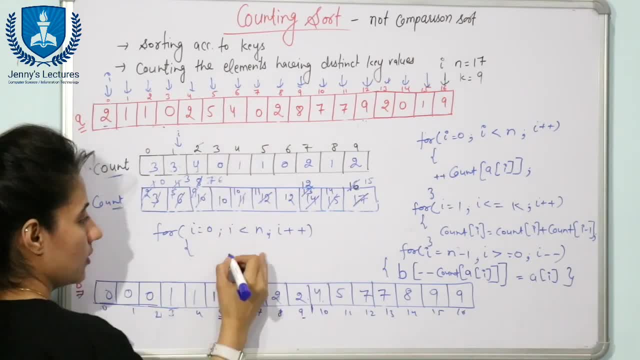 less than equal to n minus one. less than equal to n minus one. i plus plus. just copy the content here. i plus plus. just copy the content here. i plus plus. just copy the content here: array name is array. name is array. name is a. we are going to copy the content of b. 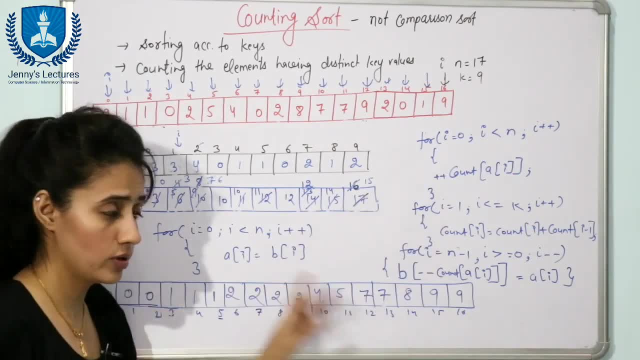 a. we are going to copy the content of b. a. we are going to copy the content of b into into into a. this is how we are going to code this a. this is how we are going to code this a. this is how we are going to code this thing. 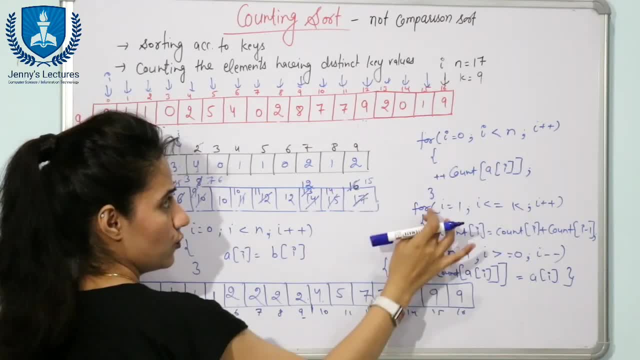 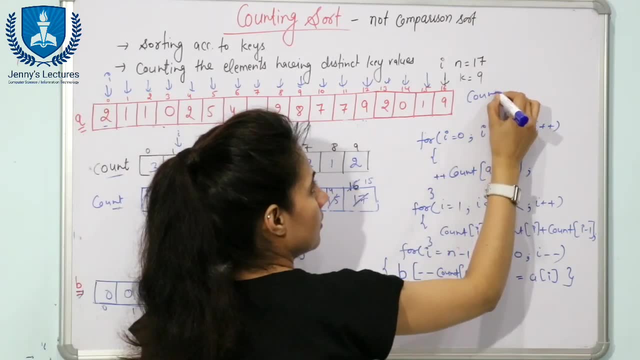 thing thing. fine, this the logic, this logic, these fine, this the logic, this logic, these fine, this the logic, this logic, these four, four, four maybe count. so in count sort you can maybe count. so in count sort you can maybe count, so in count sort you can pass. 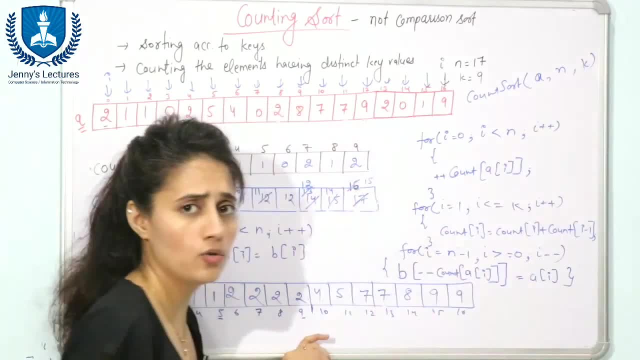 pass, pass array. or you can say the number of array, or you can say the number of array, or you can say the number of elements, and sometimes k value would elements and sometimes k value would elements and sometimes k value would also be passed. also be passed. also be passed, it is given. then you can pass the k. 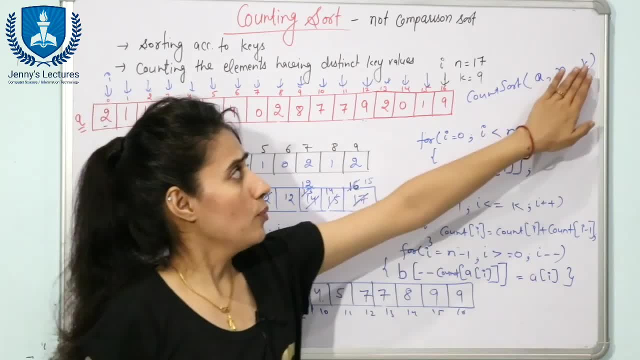 it is given, then you can pass the k it is given, then you can pass the k value, value value- fine, or if you will not pass the k, fine, or if you will not pass the k, fine, or if you will not pass the k value. here you can calculate within this: 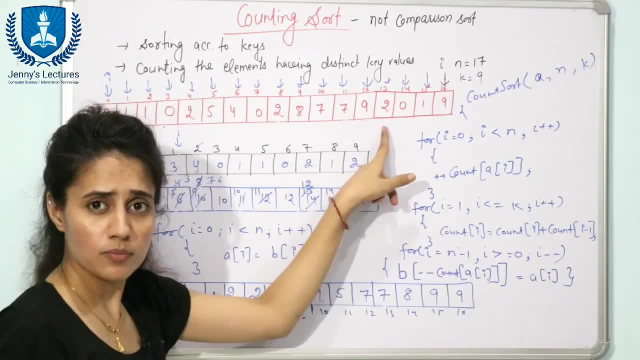 value. here you can calculate within this value. here you can calculate, within this function. you can calculate the k value function. you can calculate the k value function. you can calculate the k value. just find out the maximum. just find out the maximum, just find out the maximum element from the given array that could. 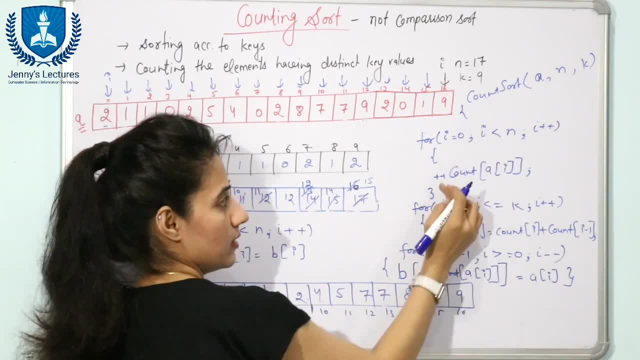 element from the given array. that could element from the given array. that could be the k value, be the k value, be the k value. fine, and just take. fine, and just take fine, and just take initializer array count. i guess you can. initializer array count, i guess you can. 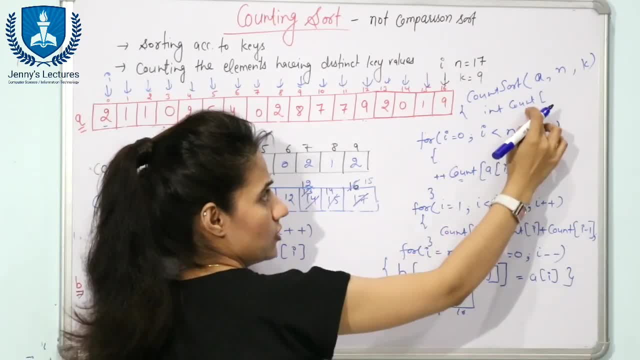 initializer array count. i guess you can take this one, this, take this one. this, take this one. this, sorry, the size would be k plus one. sorry, the size would be k plus one. sorry, the size would be k plus one. something like this: take another array. something like this: take another array. 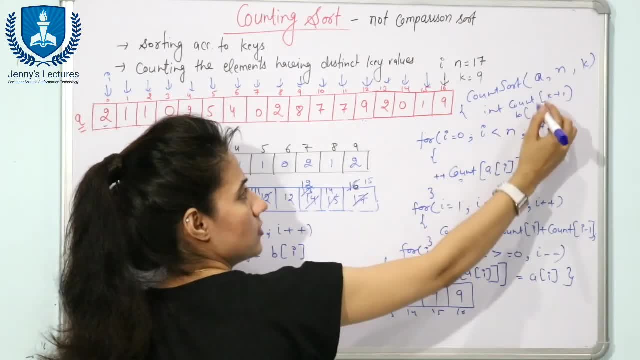 something like this: take another array: that is b, that is b. that is b. and the this b would be same as, and the this b would be same as, and the this b would be same as the size of original array if n elements. the size of original array if n elements. 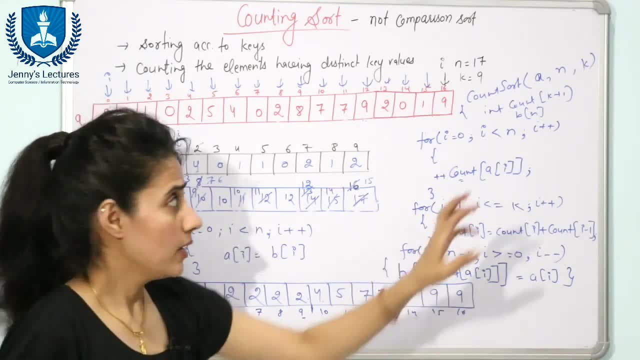 the size of original array. if n elements, then b of n, something like this. so i then b of n, something like this. so i then b of n, something like this. so i guess you can write down this count. guess you can write down this count. guess you can write down this count: sort, initialize or declare this count. 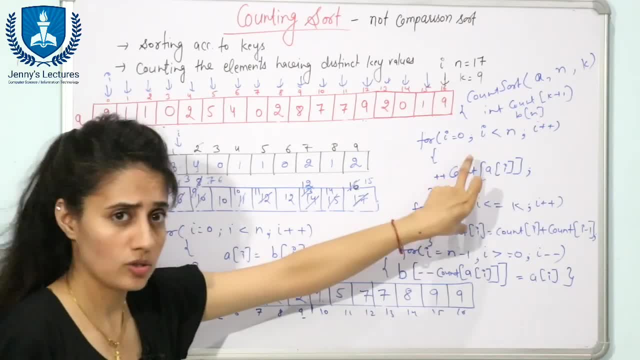 sort, initialize or declare this count. sort, initialize or declare this count, array or array, or array or b array, something like this: this is the b array. something like this: this is the b array. something like this. this is the main logic, these four main logic, these four main logic, these four, four loops, and just call. 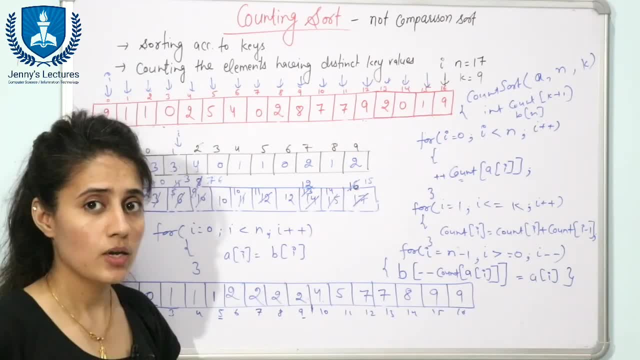 four loops and just call four loops and just call this count sort function into main, this count sort function into main, this count sort function into main function. see now what is the time function. see now what is the time function. see now what is the time complexity for this count sort. 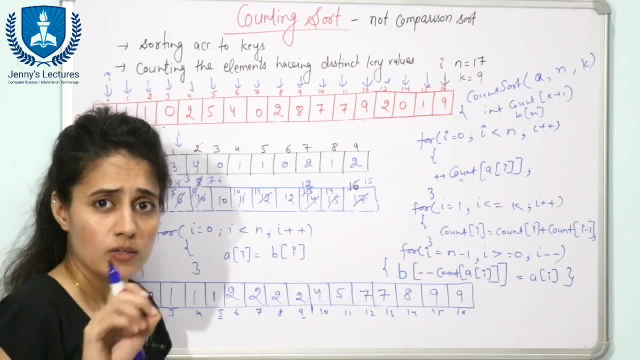 complexity for this count sort complexity for this count sort time. complexity would be what see time time complexity would be what see time time complexity would be what see time. complexity is what complexity is what complexity is what. just find out the calculations. just find out the calculations. just find out the calculations for the four loops. 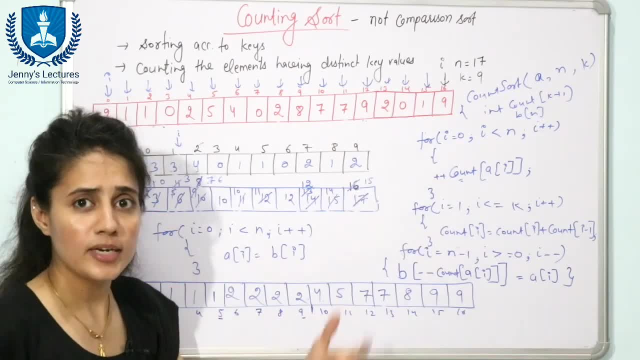 for the four loops, for the four loops given in the program. how many four loops given in the program? how many four loops given in the program? how many four loops: one, two, three, four. one, two, three, four. one, two, three, four. how many times the statements written? how many times the statements written? 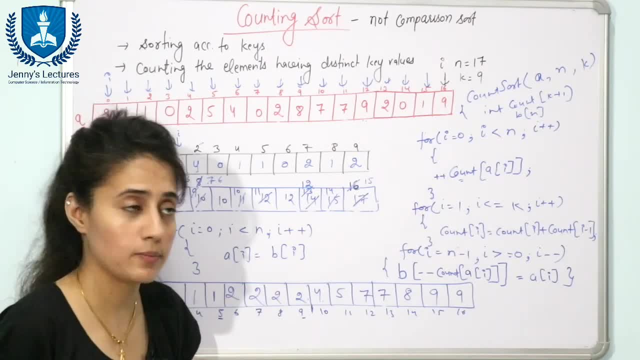 how many times the statements written within the four loops, within the four loops, within the four loops, has been executed. how many times see has been executed? how many times see has been executed? how many times see this for loop? this statement has been this for loop? this statement has been. 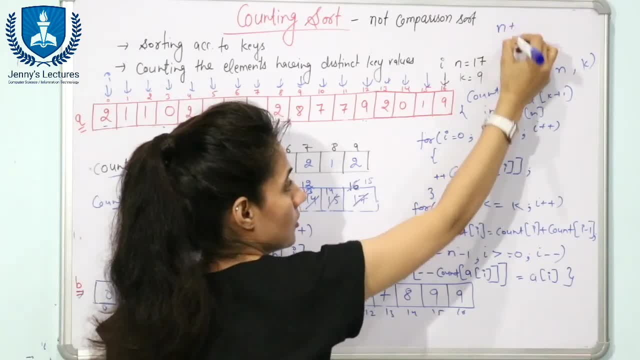 this for loop. this statement has been executed for n times. executed for n times. executed for n times: fine n times. plus this for loop: k times: fine n times plus this for loop: k times: fine n times plus this for loop: k times. this for loop, also n times. 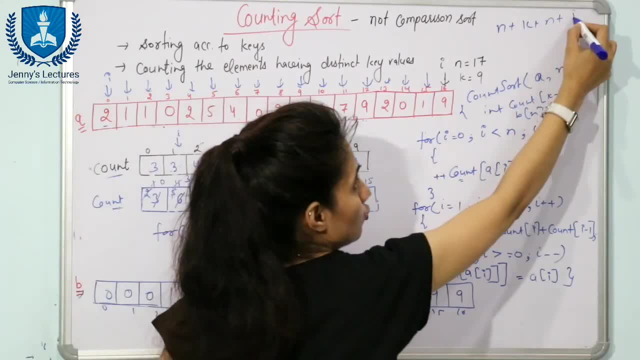 this for loop also n times. this for loop also n times. and this for loop also from 0 to n. and this for loop also from 0 to n. and this for loop also from 0 to n means n times means n times, means n times. so maybe something like this: 3n plus k. 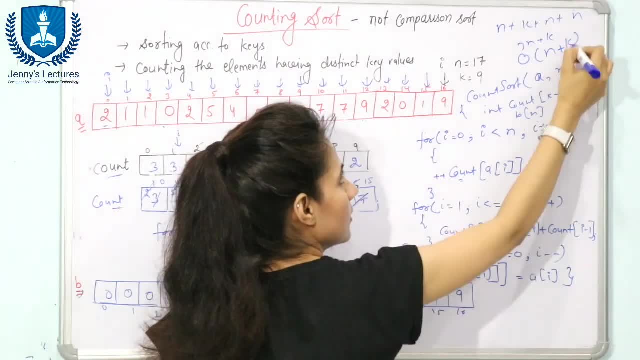 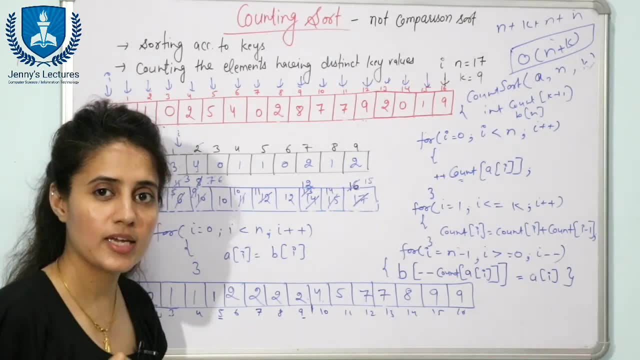 so maybe something like this: 3n plus k, so maybe something like this: 3n plus k, or you can say, or you can say, or you can say: order of n plus k. this would be the time complexity, this would be the time complexity, this would be the time complexity: n plus k. where k is given the range. 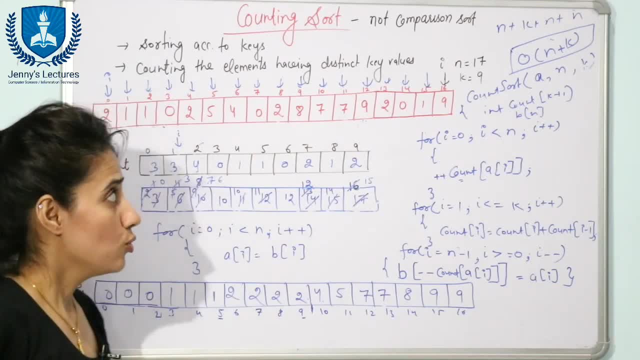 n plus k where k is given the range. n plus k, where k is given the range n is number of elements in the array. n is number of elements in the array. n is number of elements in the array. so so so if k is suppose a constant, you can say: 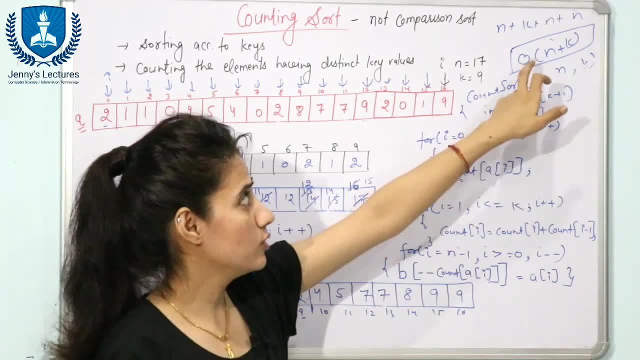 if k is suppose a constant, you can say: if k is suppose a constant, you can say so. so so you can neglect this k and you can say you can neglect this k, and you can say you can neglect this k and you can say order. of order of. 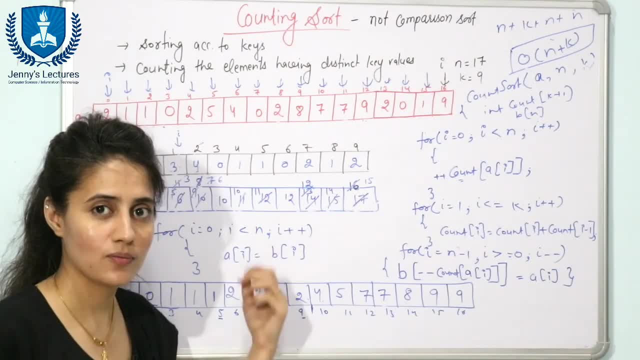 order of n in linear time. you can sort n in linear time. you can sort n in linear time. you can sort the elements. one drawback of this: count the elements. one drawback of this: count the elements. one drawback of this: count. sort algorithm can be say this: sort algorithm can be say this: 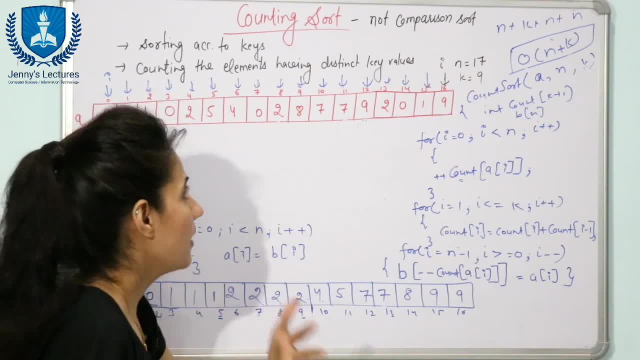 sort algorithm can be say this: k value should be feasible, k value should be feasible, k value should be feasible. what does that mean? let us suppose you. what does that mean? let us suppose you. what does that mean? let us suppose you, are you are taking an. are you are taking an? 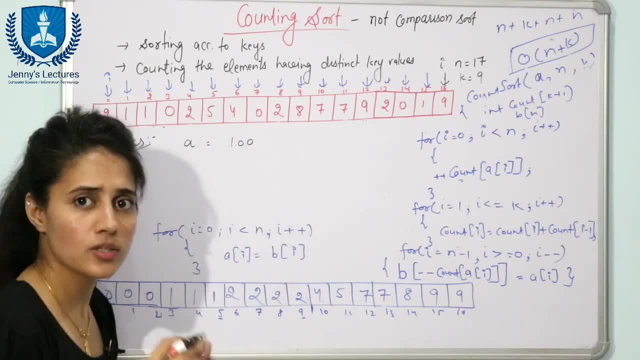 are. you are taking an array a and having array a and having array a and having 100 elements in the array. here we have 100 elements in the array. here we have 100 elements in the array. here we have taken 17 only, taken 17 only. 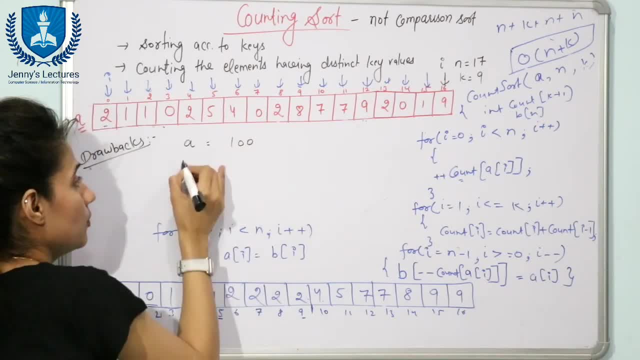 taken 17 only, and in that array we have 100 elements, and in that array we have 100 elements. and in that array we have 100 elements. and let us suppose k value is, and let us suppose k value is, and let us suppose k value is 10 000. 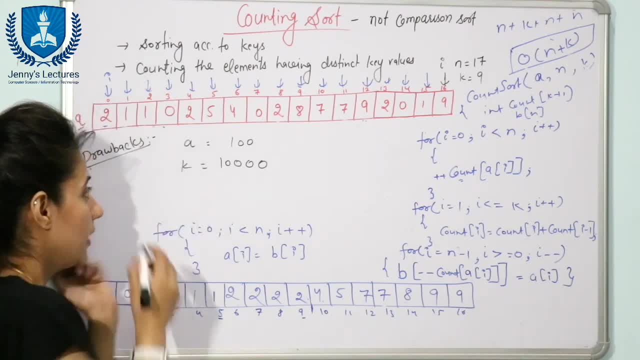 10 000, 10 000. now, what will happen now? what will happen now? what will happen? you are going to create a. you are going to create a. you are going to create a count array and the size of this count count array and the size of this count. 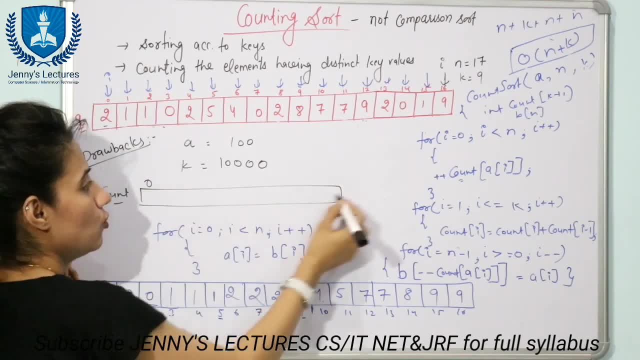 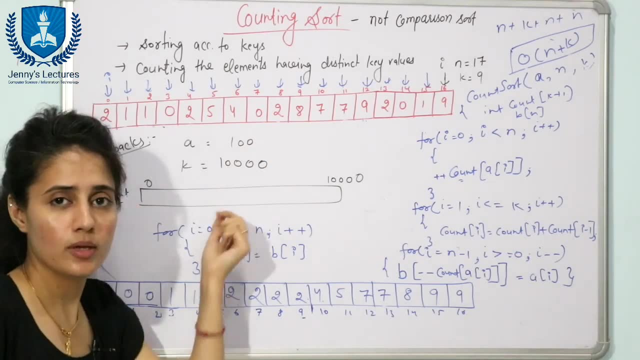 count array and the size of this count array would be, array would be. array would be: how much from zero to how much from zero to how much from zero to ten thousand, ten thousand, ten thousand. in these locations, only in these locations, only in these locations, only hundred elements would be there, only. 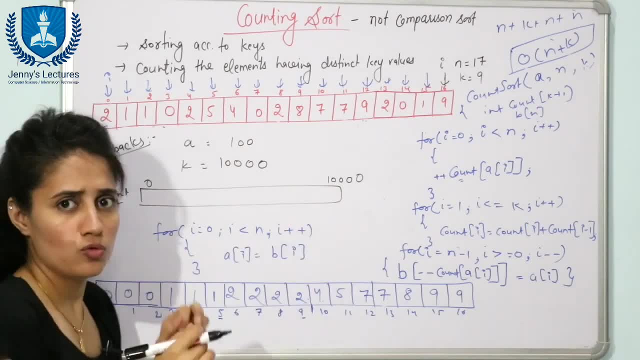 hundred elements would be there. only hundred elements would be there, only hundred elements. so many, many places in hundred elements, so many many places in hundred elements. so many many places in this count sort would be zero, zero, zero. this count sort would be zero, zero, zero. this count sort would be zero, zero, zero, zero. something like this: 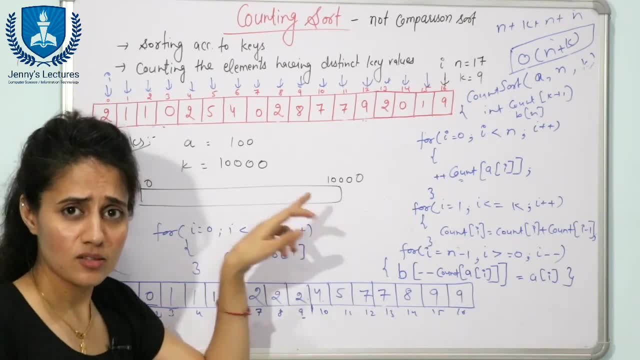 something like this, something like this: fine, so this should not be a case in fine, so this should not be a case in fine, so this should not be a case in this case, this applying of this count, so this case, this applying of this count, so this case, this applying of this count, so it is not feasible. 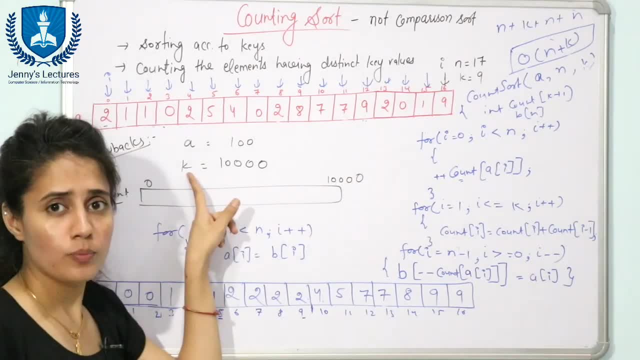 it is not feasible. it is not feasible, fine. so the upper bound, the upper bound, fine. so the upper bound, the upper bound, fine. so the upper bound, the upper bound, for this k should be, this k should be for, this k should be, this k should be for, this k should be, this k should be. order of. 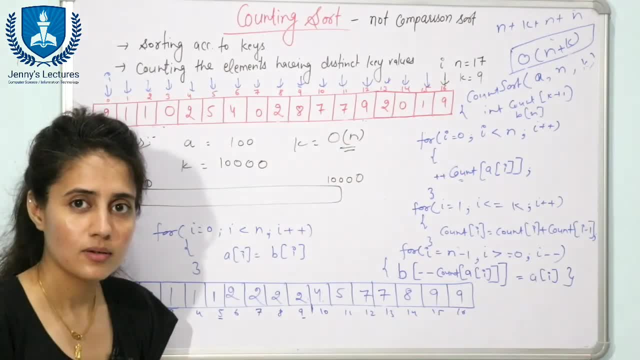 order of order of n. n means number of elements in the array. upper limit for this k would be number of upper limit for this k would be number of upper limit for this k would be number of elements in the number of elements is. elements in the number of elements is. 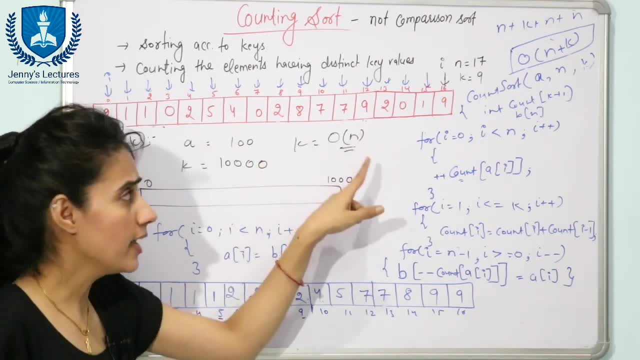 elements in the number of elements is 100, 100, 100, then k can be 100, then k can be 100, then k can be 100. it's not like it can be 100, it can be 2n. it's not like it can be 100, it can be 2n. 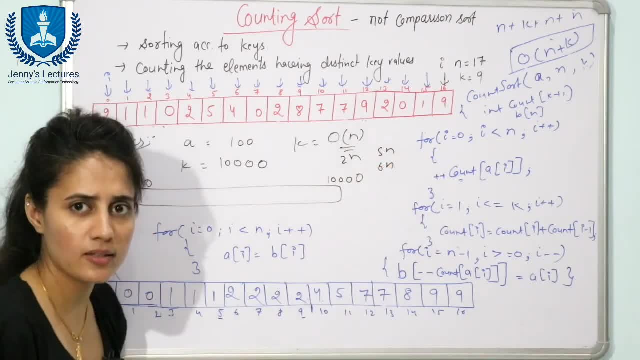 it's not like it can be 100, it can be 2n, it can be 5n, it can be 6n, something like it can be 5n, it can be 6n, something like it can be 5n, it can be 6n, something like this, but it cannot be. 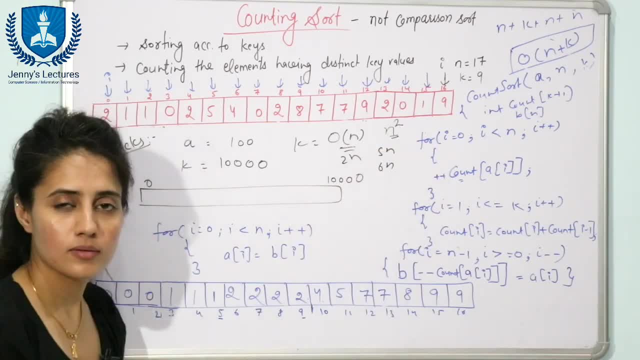 this, but it cannot be this, but it cannot be approximately n square. fine, so this is the bound for this k, this fine, so this is the bound for this k, this fine, so this is the bound for this k. this k should be order of k should be order of. 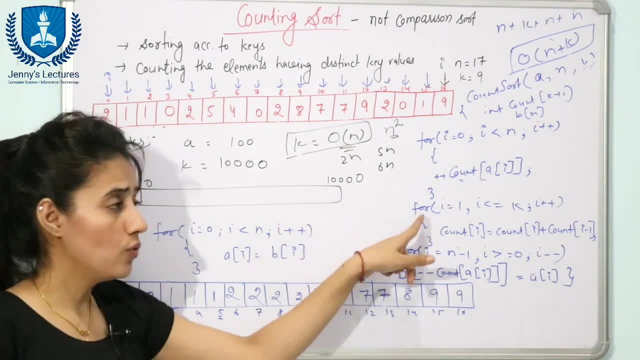 k should be order of n. and second topic is this: count sort n. and second topic is this: count sort n. and second topic is this: count sort will not work for negative values and will not work for negative values and will not work for negative values and floating point values. 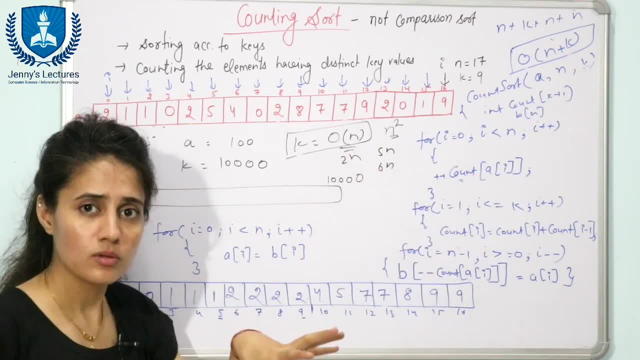 floating point values. floating point values. you can modify this count sort for you can modify this count sort for you can modify this count sort for negative values. after modify negative values. after modify negative values. after modify modification. it can work, maybe you can modification. it can work, maybe you can. 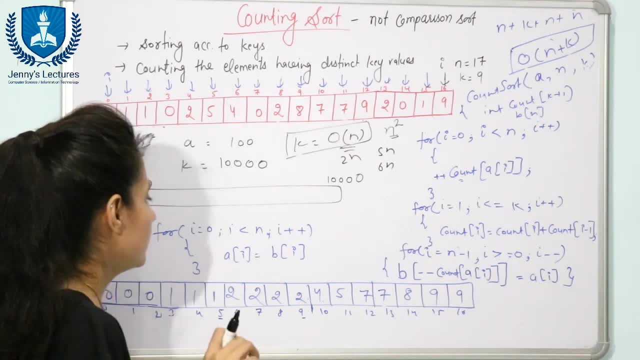 modification. it can work. maybe you can apply some normalization methods, apply some normalization methods, apply some normalization methods like see, like, see, like see minus negative values are there. so how minus negative values are there, so how minus negative values are there. so how you can normalize this, how you can apply. 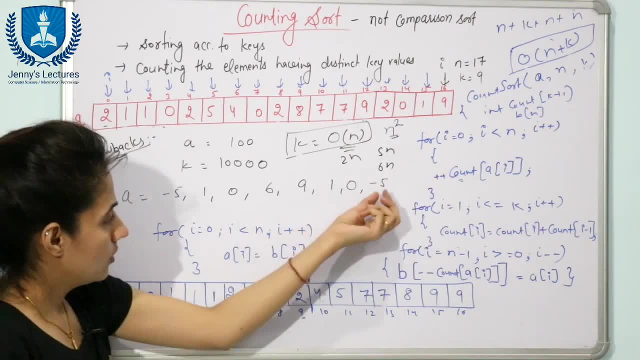 you can normalize this, how you can apply. you can normalize this, how you can apply, how you can modify this count. so how you can modify this count, so how you can modify this count. so just find out. this minus value is 5, so just find out, this minus value is 5, so 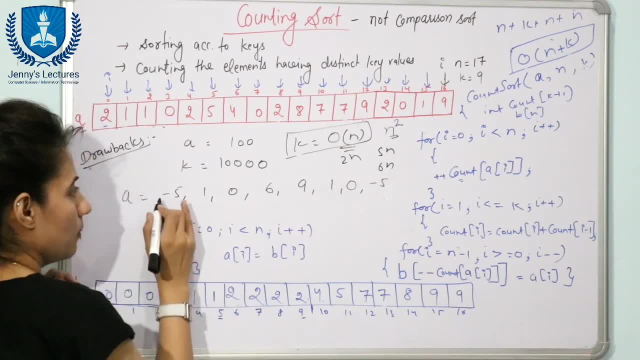 just find out, this minus value is 5. so just add this 5 to all the values. just add this 5 to all the values. just add this 5 to all the values minus 5 plus 5. 0 plus 5, 6 plus 5. 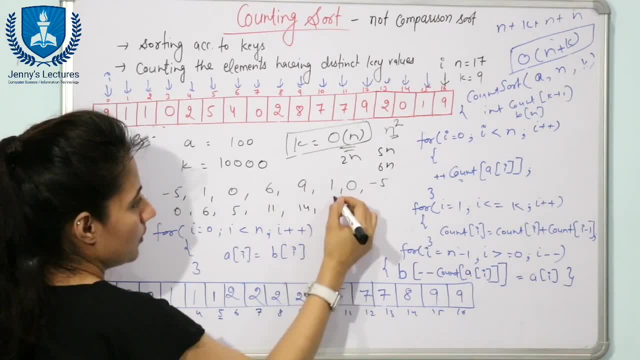 minus 5 plus 5, 0 plus 5, 6 plus 5 minus 5 plus 5, 0 plus 5, 6 plus 5, 5 plus 5, 11 plus 5, 5 plus 5, 11 plus 5, 14 plus 5 is 6 plus 5 is 5, and here we: 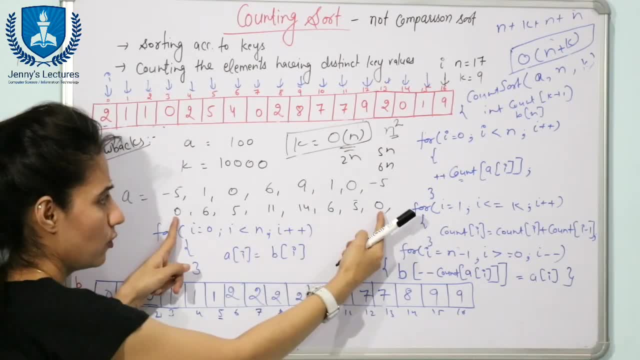 14 plus 5 is 6, plus 5 is 5. and here we: 14 plus 5 is 6 plus 5 is 5, and here we have zeros now. this is the array the have zeros now. this is the array the have zeros now. this is the array. the range would be here is c, from 0 to. 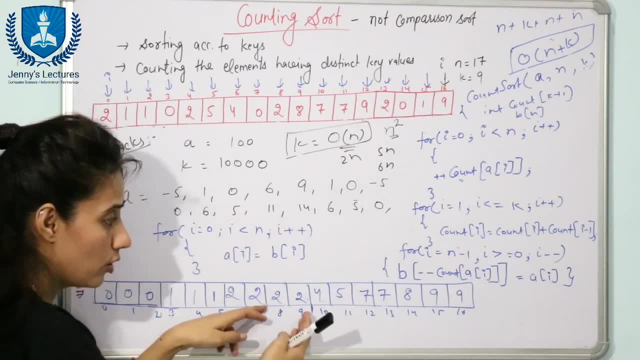 range would be here is c from 0 to. range would be here is c from 0 to 14. you can say 14, you can say 14. you can say fine, and again after sorting, you can fine, and again after sorting, you can fine, and again after sorting, you can again decrement this. you can again do. 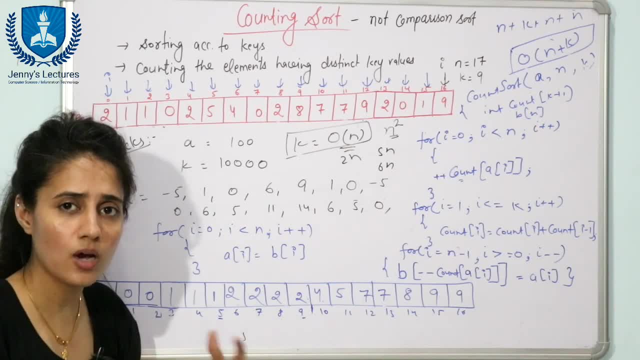 again, decrement this. you can again do again, decrement this. you can again do minus 5 from the result, minus 5 from the result, minus 5 from the result. so this is how you can, so this is how you can, so this is how you can normalize the negative values and you 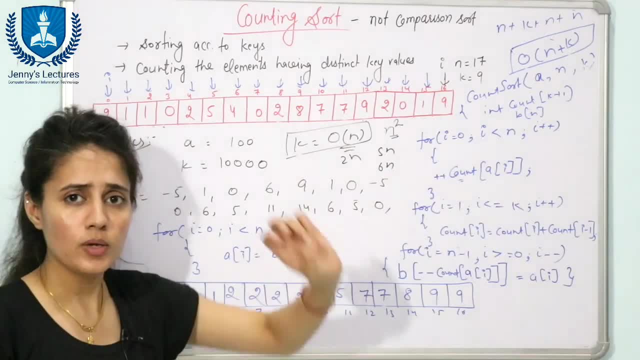 normalize the negative values and you normalize the negative values and you can apply this count sort, can apply this count sort, can apply this count sort. but this logic directly cannot be, but this logic directly cannot be, but this logic directly cannot be applied on negative values and floating. 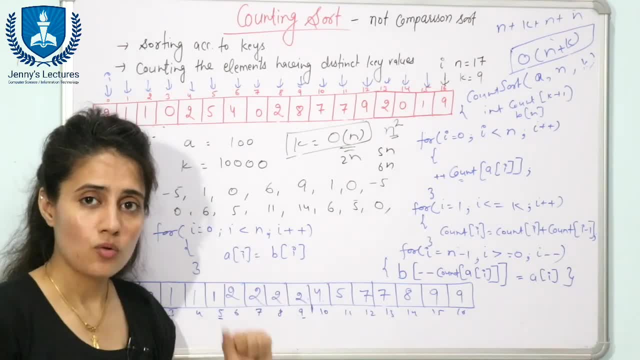 applied on negative values and floating applied on negative values and floating point values. point values, point values plus one more drawback of this count plus one more drawback of this count plus one more drawback of this count. sort is what sort is what sort is what? it cannot be applied if the values are. 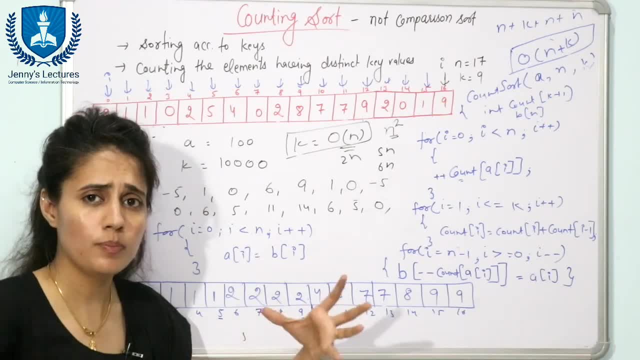 it cannot be applied if the values are. it cannot be applied if the values are different in any range. there is no different in any range. there is no different in any range. there is no proper or specific range: see the values. proper or specific range: see the values.